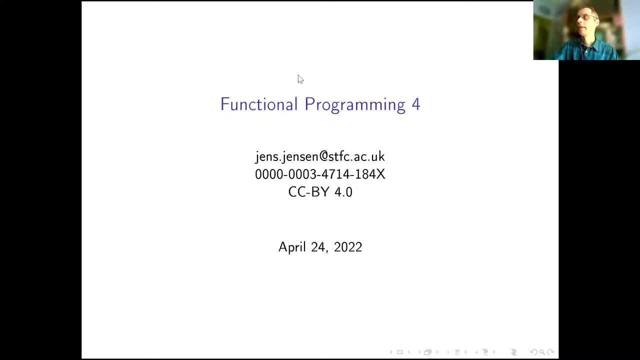 This is very much a personal perspective, but Lisp was the second programming language I learned, The first one having been some sort of tiny computer basic or some such. So I have been programming Lisp for a while, and Emacs as well, I am actually so. my natural home, if you like, is common Lisp rather than Emacs Lisp. 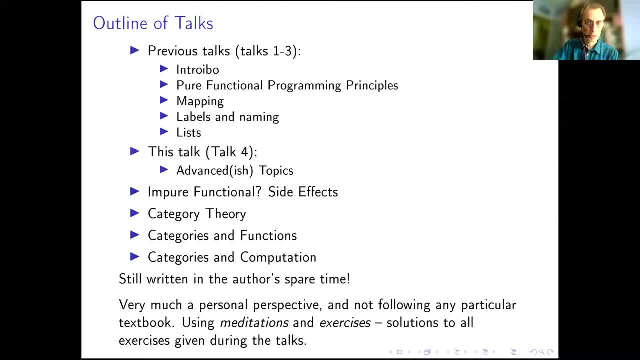 Okay, so let's see what we can do today. This is sort of a general overview of the talks. The previous talks, as David mentioned, are still available. They've been recorded somewhere. You can see the slides. This talk is what I sort of call advanced topics, though you might disagree, I think, or we'll see. 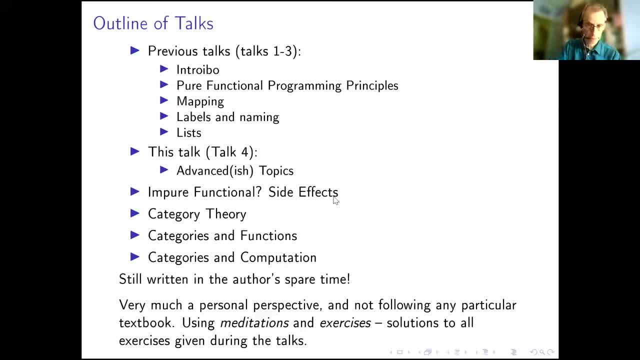 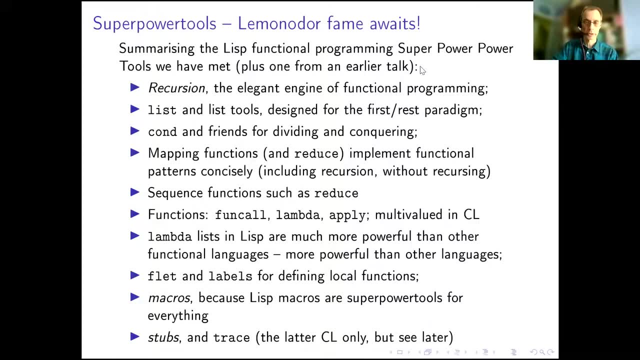 And there will be more stuff to come later And it is very much a personal perspective on using Lisp for functional programming. So, summarizing, to summarize the first three talks in a single slide, This is sort of the superpower tools that I thought. 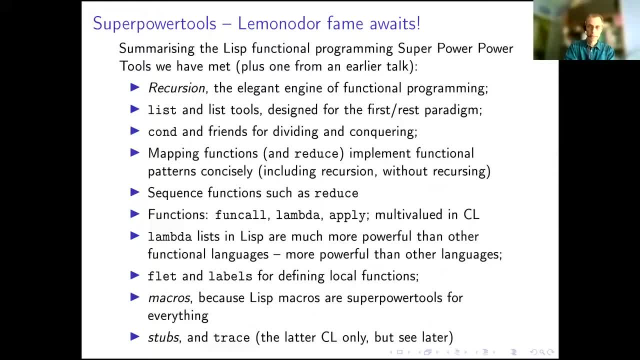 I would want to try to identify that are available in Lisp for functional programming and make things really nice. Exam mapping functions actually implement many of the common paradigms that you would normally use recursion for, But obviously they don't recurse because they just map across lists. 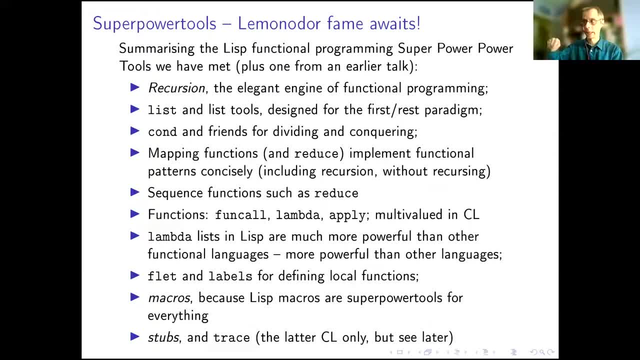 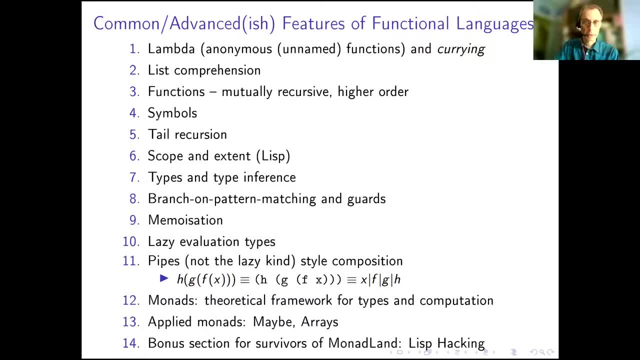 And that makes it much easier to write in Lisp because you don't get in Emacs, that you don't run out of stack or anything, even if you process large lists. So the list of what I sort of call quote unquote- advanced topics are. this list is basically here: 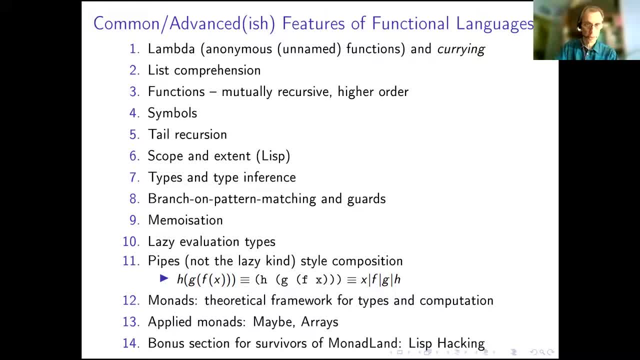 And I was planning to do the first four today And it'll be a little bit sort of a mixed bag of things, I think, because some of these topics are quite long and have a little bit of theory and stuff in them. Some of them are much shorter. 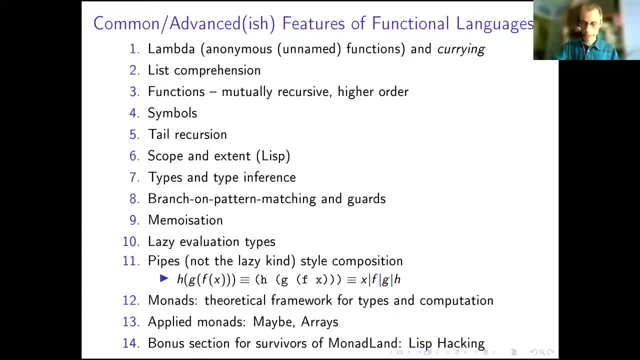 And we'll just have a bit of oh look, we've talked about this and then we can move on to something else. So five and six are slightly longer topics, and seven: I haven't finished writing yet, So we can't do those yet. 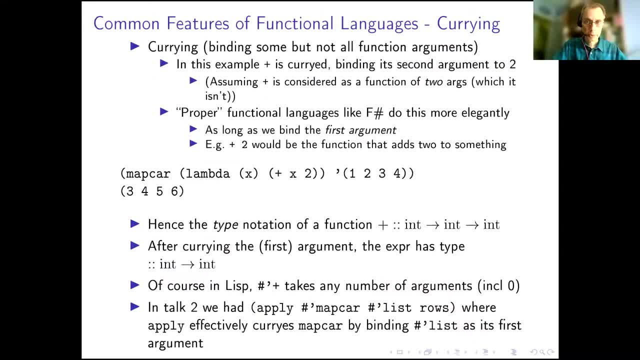 But we'll see. So let's start looking at functions and languages and stuff, because we know functions take arguments and arguments. You can have zero arguments, You can have one argument or two arguments. So for a moment let's think of plus as a binary function. 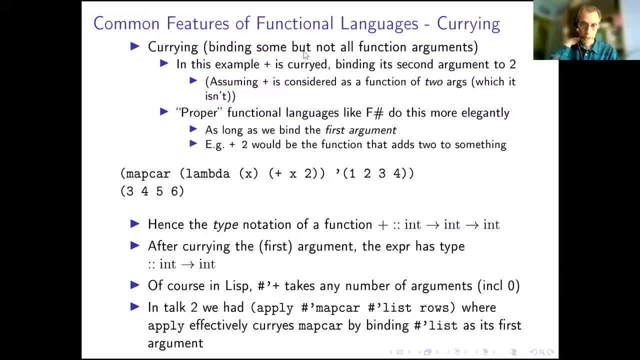 It takes precisely two arguments, And those arguments are obviously numbers, So I'm trying to get rid of this zoomy thing on my screen. So imagine that plus is a binary function and then we give it one parameter, one argument, the other one. 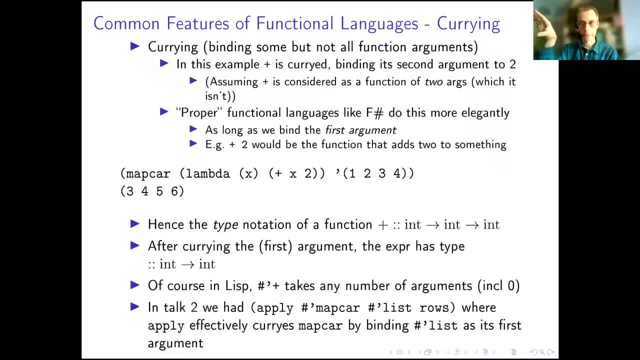 So if I just say plus two in a normal functional language, then it will bind two to one, to the first Argument, to plus, And the other one is still unbound. So effectively. what I get is a function of one variable, namely a function which adds two to something. 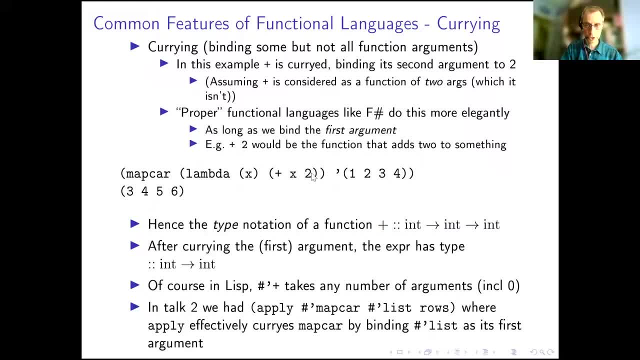 If I want to say that in Lisp, I have to say lambda x plus x two, because that is then the most concise way I can express a function that adds two to some number. So I can express that as a function of a single variable. 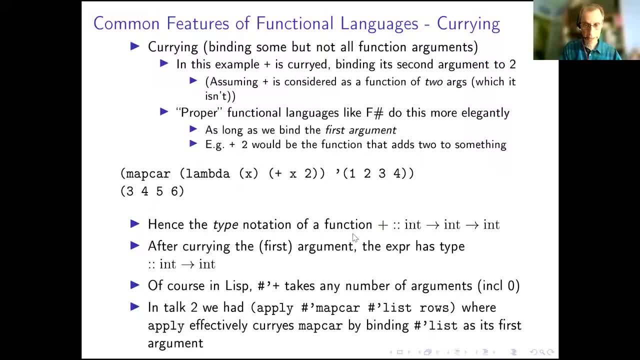 So in functional programming you will often find the notation of a function. It will say plus, and it will say one colon or two colons- The notation varies a bit from one author to the other- And then it will say int, arrow, int, arrow, int. 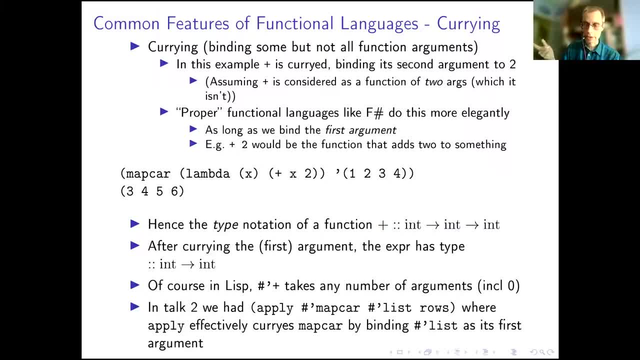 And the idea behind that is that plus itself is a function which, if you give it one integer, then it returns. a function that takes an integer and returns an integer, Like the one that adds two to something. If you give it two integers, then you just get an int back. 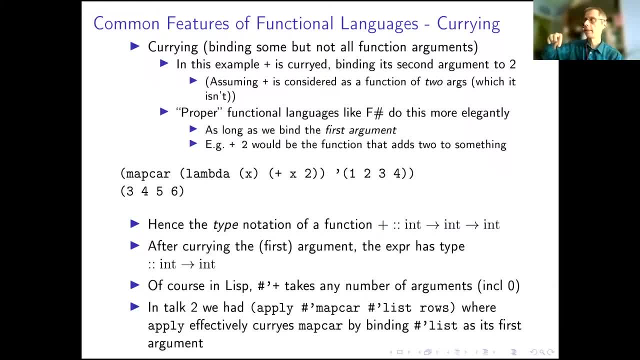 So the notation is there to say that you can sort of fill up the arguments to the functions one at a time by binding them one at a time. In functional languages you normally bind them with the first argument first and then the second argument and then the third argument until the function has all its arguments. 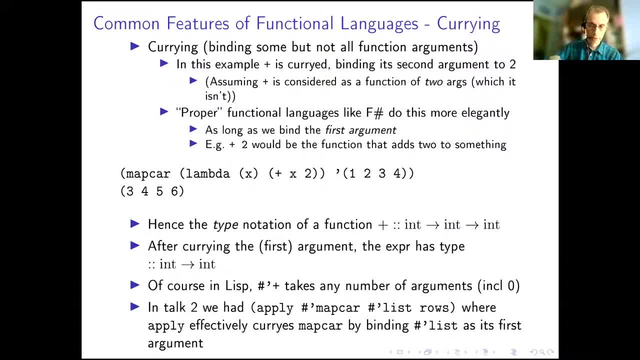 And then it can evaluate In Lisp. of course you could just bind anything you like, really, because with the plus I have actually, when I say plus x2, I have effectively bound the second argument to plus. if plus were binary. 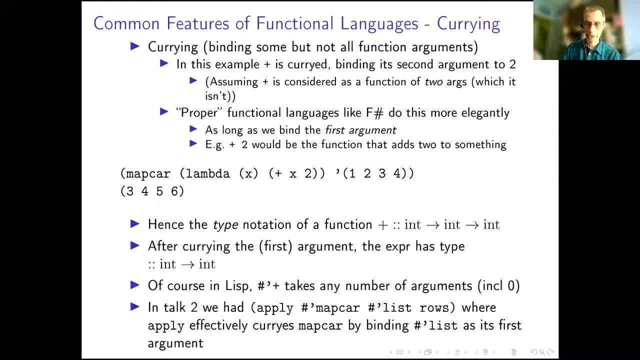 And it doesn't matter because it's just a lambda expression the way I want. So if you go and read or try to read, for example, the first argument, then you will find that it's just a lambda expression. If you go into functional papers and stuff then you will often find this: plus arrow notation: 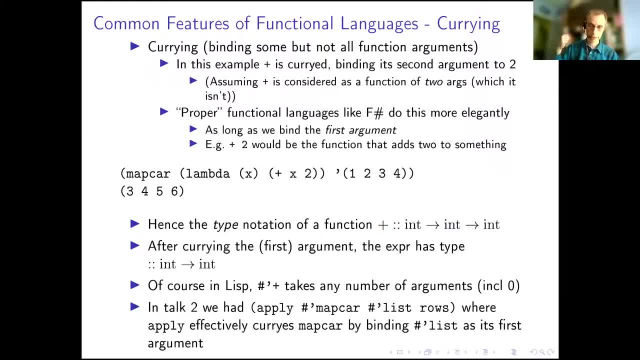 And we will probably, I think, make use of it later when we get to Monads or some such. So the notion of currying, which is named after Haskell Curry, is effectively saying that we can bind some of the arguments of a function and then we get an argument of the ones that are yet unbound, which is itself a function. 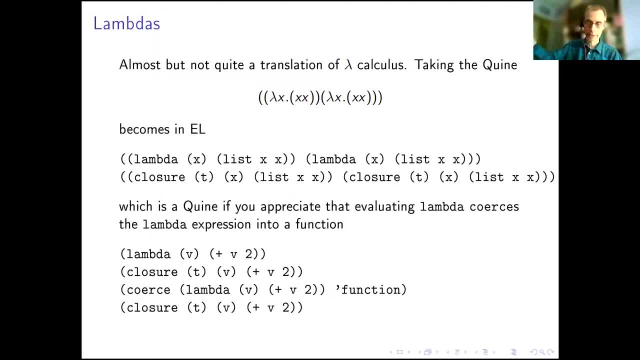 Until we have bound them all, then it can evaluate and then we get a result of some description. so in this talk I had also not planned to talk very much about lambda calculus at all, but I will just mention because we obviously we're talking about lambda sin lisp. so 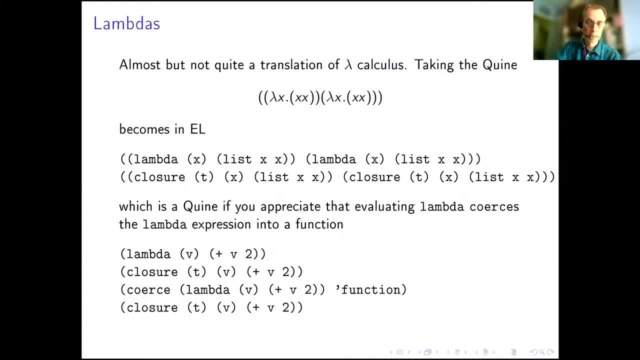 there is a collection, obviously, to lambda calculus. for example. there's an expression here on the slide where lambda X dot X. X means that it's an anonymous function that has one parameter X and if you give it a parameter X, it returns X juxtaposed with X. so X, X effectively means call X on. 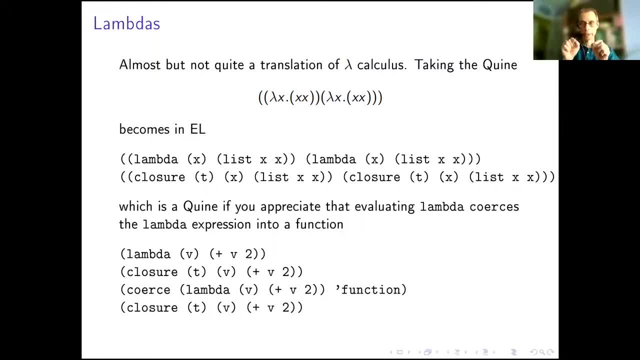 itself, because I was just putting things together in in this notation- means call the thing to the right. so the first lambda X, you of X, X, is called under second lambda X. so what it does is to take this second value and bind it to the X in the first expression and then it calls it on. 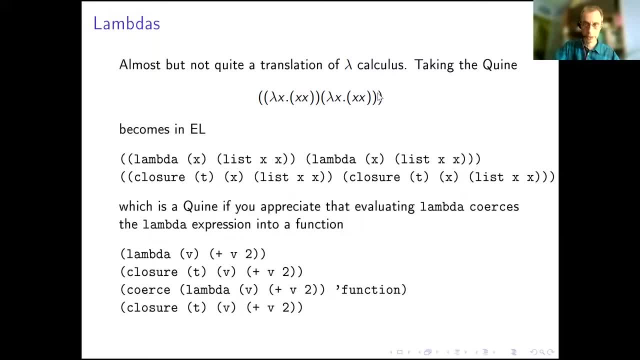 itself and you sort of get this expression out of it. and if we actually try this in the image list, we almost get the same thing. because if I just say lambda X, list X, X and lambda X, list X, X then and call that on itself, then I get. 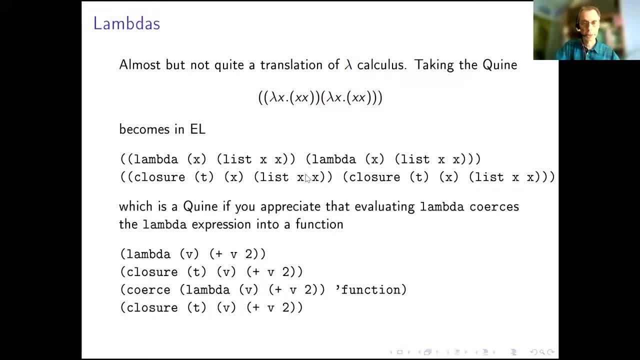 the corresponding closures. if I evaluate a lambda in eMax, I get a closure. now, list X X is not necessarily the same as phone call X X, but this was just to illustrate the expansion of the lambda list in that we actually do get something like it if I 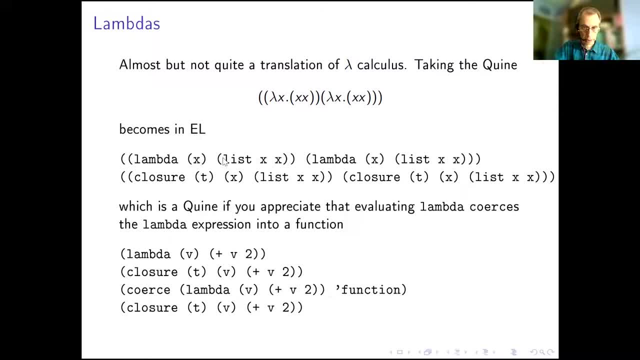 just type list X- X, then the second lambda is bound to the X in the first lambda, and then it creates the list of these. so you can see that's pretty much the same thing thing. if I then evaluate it again, then what is expressed as a list in this? 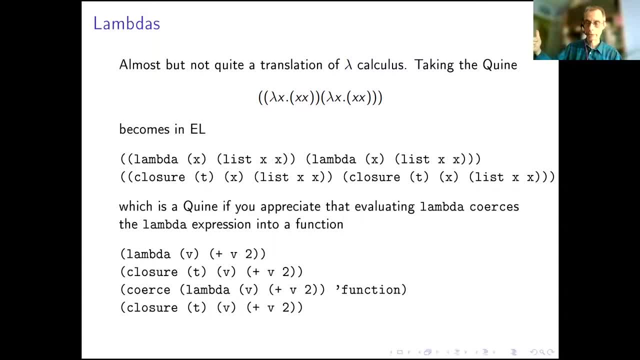 expression rather than a function call will become a function call because, as you know, the outermost list lists in lisp expresses a function call. so hopefully that's clear. that's why I've got list here rather than a function call, because the list, when I evaluate that, is a function call, it will take its 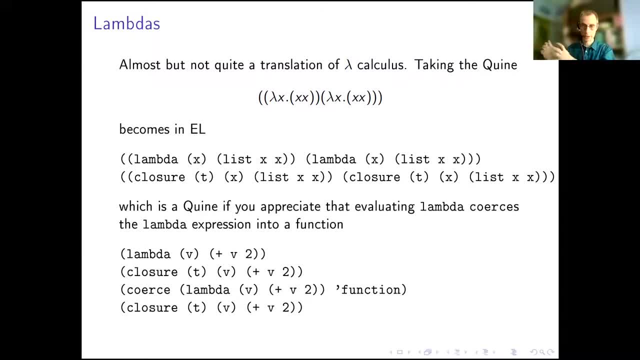 first element and call that on its second element as the argument. okay, so this is sort of more like a curiosity really, but just to say that there is a connection of some sort between the lambdas and lambda calculus. in practice, lambda expresses an anonymous function, as you know, which, when I evaluated it, 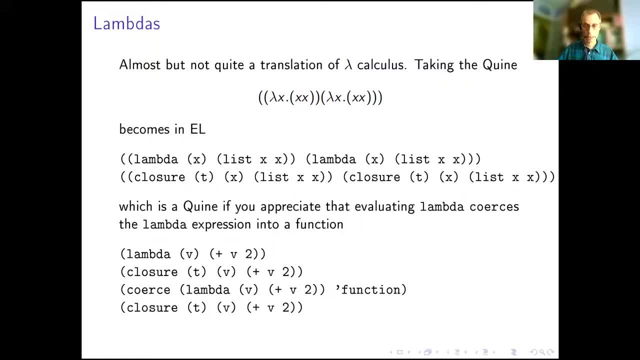 becomes a closure in a max. if I try to curse the lambda expression into a function, then the same thing will happen because it will just say, yeah, it's a closure. so technically the lambda isn't really a function, but in every, almost every context you can think of, it will behave as if it were a function because it gets. 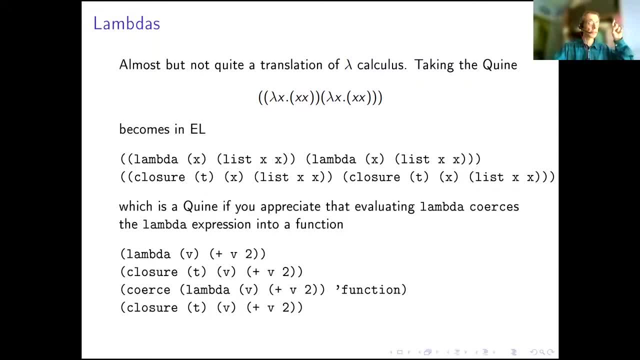 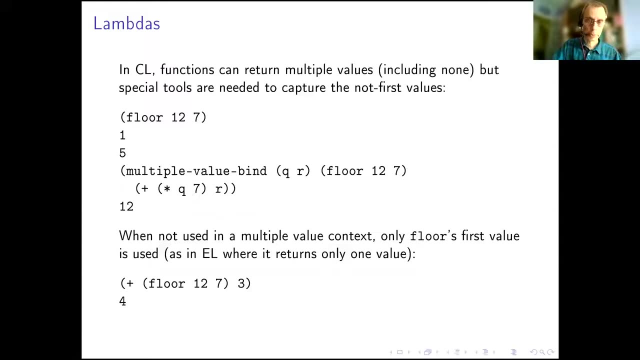 cursed to a function if it's found in the first as the first item in a list, like where the function should be. so the other thing: I won't go into this too much, but I just thought it's worth mentioning that in in common listeners. there are a number of ways that you can use the function call to call a function call. so the other thing: I won't go into this too much, but I just thought it's worth mentioning that in in common list. 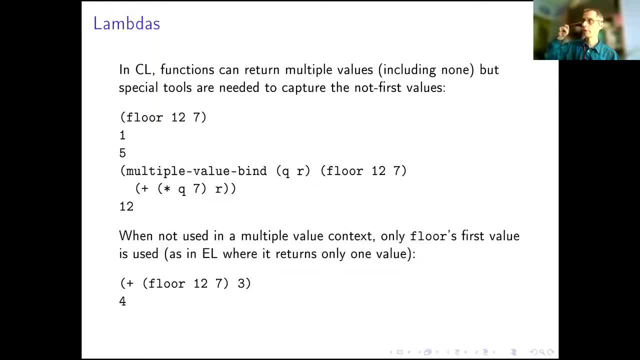 functions can return multiple values. so in a max list, functions always return precisely one value, and in functional programming that is normally what you see. functions return precisely one value. but in common list functions can actually return any number of values, from zero to an implementation specific maximum, which is usually quite high. the thing is that while functions 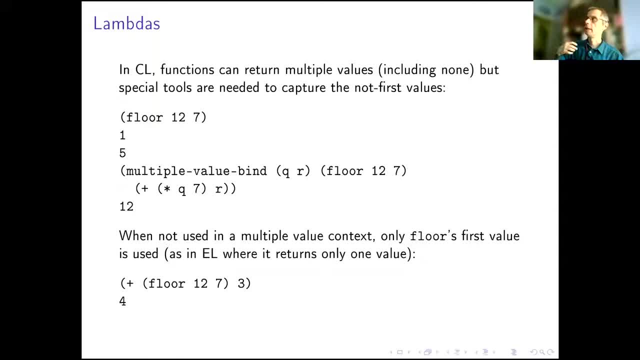 can return multiple values. normally it is only ever the first one that gets used. if you want to use all of all of the values returned by the function, you have to use a special construction like this multiple value point. so in common list, for example, floor returns the quotient. 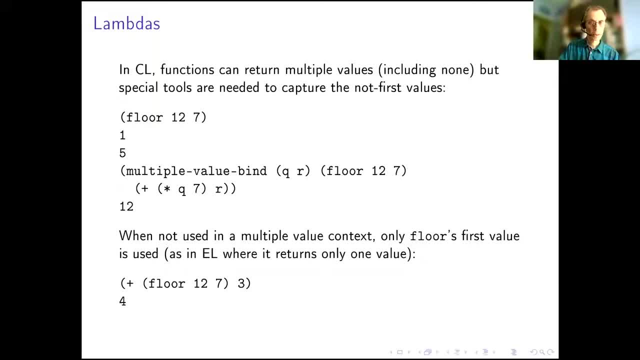 and the remainder of integer division in emacs. this bit doesn't. it will just return the quotient. but then in a normal context in common list, if you wanted to use the floor function, you will just get the first value and you know the second value will be ignored. if you wanted to use the 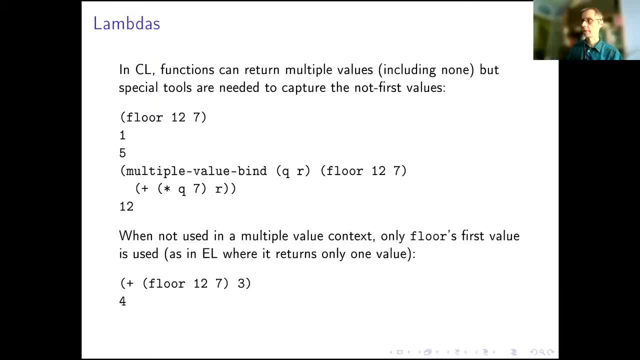 to capture the second value, because you have a some large integers perhaps, and the calculation is slightly expensive and you might as well calculate the quotient that remained at the same time, because you because you're doing euclid's algorithm or something, then you would need to use multiple value bind to capture those and that's like a handful of multiple value. 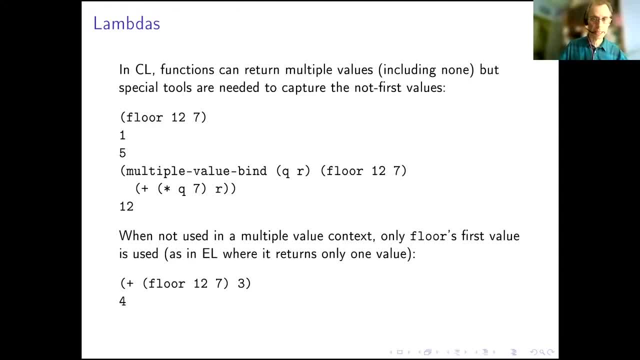 constructions that can access the the subsequent values returned by a function. but even in common list, if i say plus floor 12, 7 and then 3 flaws, 5, 7 will give me one and the remainder value, 5, will get ignored, because if i wanted to use it, i would need to use one of these multiple value. 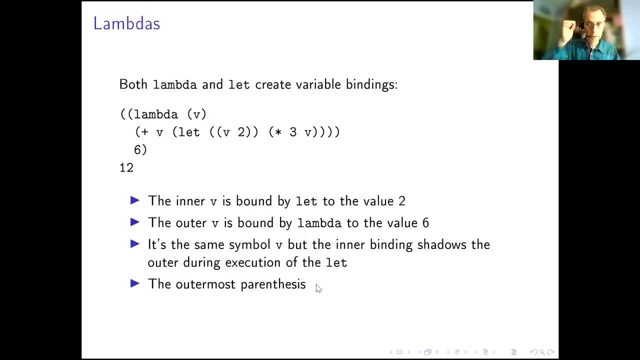 constructions. the other thing to note, if you just think two slides back when we talked about lambda calculus: the lambda x and then x dot x, um, the the first of those had a value substituted into it. so in fact lambda creates a binding, just like lead does. if i have a lambda expression here, 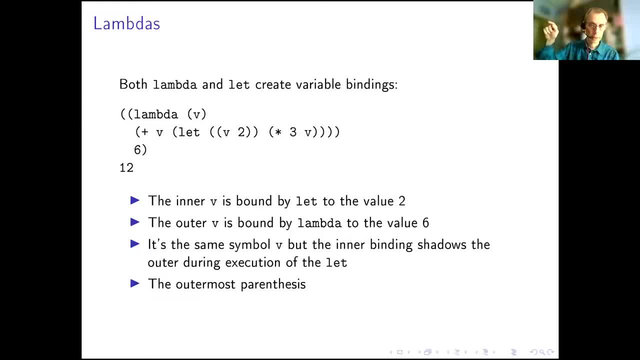 that is now the first part of the list, so it gets evaluated then that v will be bound to the whatever i pass in as the argument to the function, which in this case is six, and inside the function, in the body of the function, there's an expression plus v. 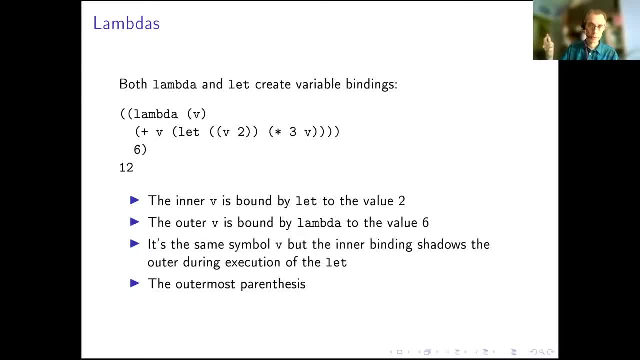 and then another lead that binds v again. so there are now the same symbol. v represents a variable in both cases, but it has different bindings. the innermost binding is created by let and will bind v to 2, and 3 times 2 is 6.. 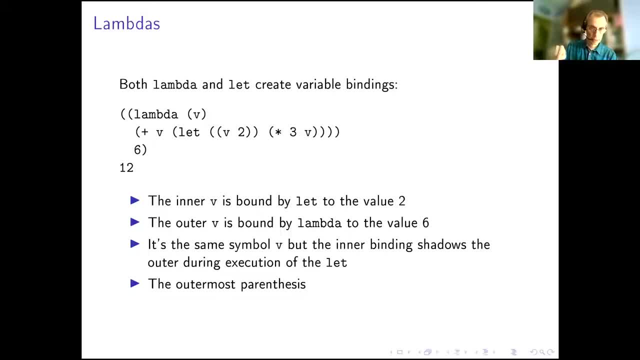 the outermost binding is set by the function call in the lambda expression, and the binding here is is: v is bound to 6, so you get 6 plus 6, which is 12.. i know there's a dangling sentence here at the end. i'm not sure what i was trying to say. i was trying to remember but i can't. 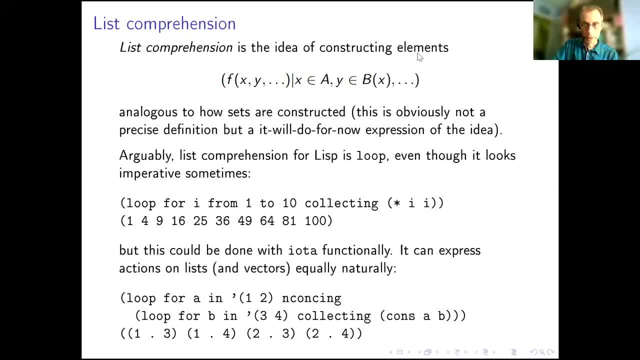 remember. so, moving on, um list comprehension is another one of the things that people talk about for functional programming. uh, because you express the kind of list you want to build and what you want to build out of, and then your language happily starts constructing that list for you. 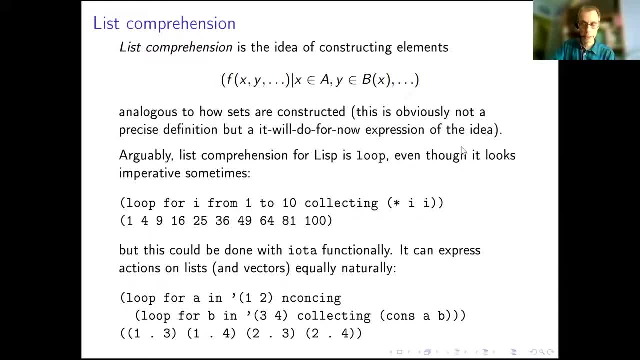 now i would argue that loop is list comprehension in lisp and you're probably thinking that loop for i from one to ten, collecting the square phi is a very imperative way of writing things. it's like a full loop. but if you really wanted to iotad, so you could loop for i in iota 10 or whatever, and you could. 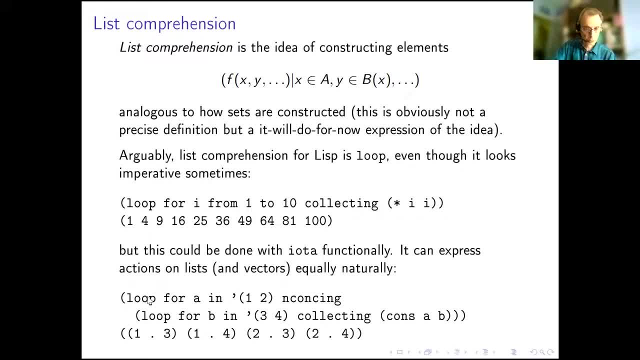 use that. if you use the more advanced constructions like loop for a list, and then you you concatenate the the lists that you'll write for a list. you- i think you've already written that- create that you get by collecting a and B comes together, then you can see it actually takes one from the first list and picks ones from the other list and personally actually get all the pairs, which is what you want to list. list comprehension. 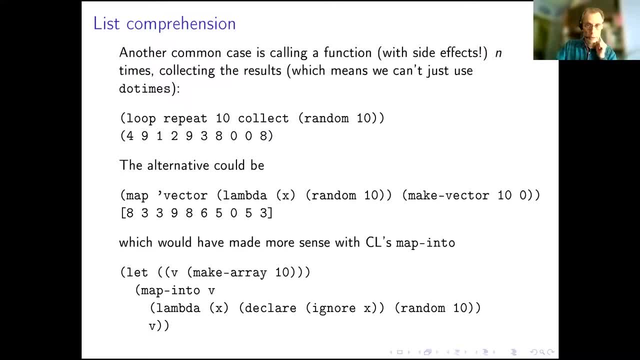 The other thing you might want to do: if you have a function that has side effects and you want to call it several times because you want to see what those side effects are or what happens if you're generating random numbers or something, then whoops. 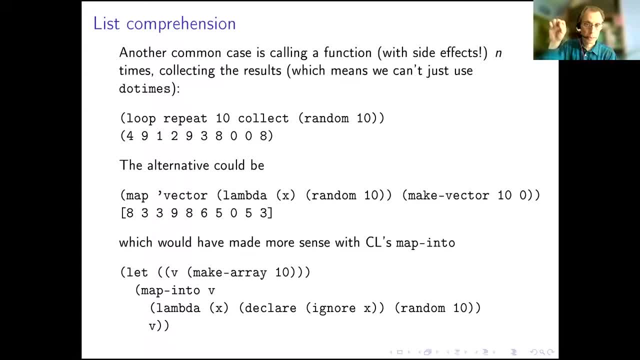 Sorry, wrong button. Then the easier ways to say loop, repeat 10 times, collect whatever those random numbers are, Rather than creating a vector of length 10 and And mapping stuff into it or something which looks a little bit artificial, if you, if you're a purist, you want, you may want to say 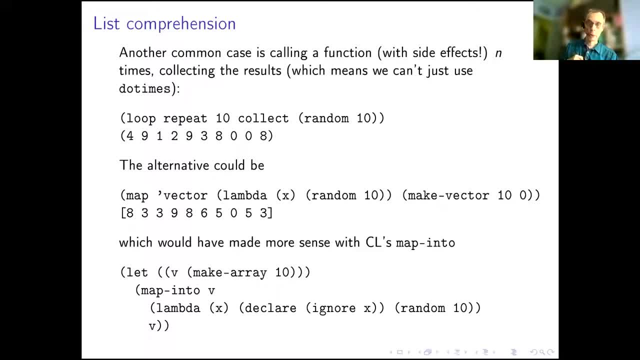 Well, I really want to use functional languages. I don't want to write for, but In my opinion, just using loop for these kind of things is actually quite like this list comprehension, and list comprehension is apparently considered quite functional, so so there's not too bad. 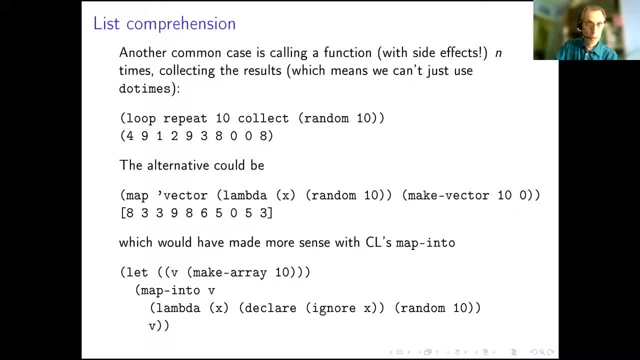 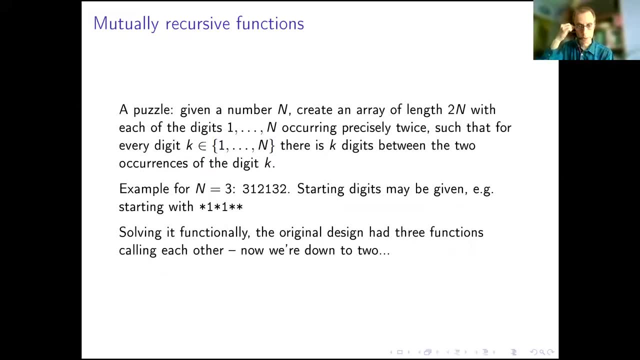 But it's not necessarily a good idea to use functional languages, but it's a good idea to use functional languages, which are not necessarily the best. The one other thing I wanted to- as I know, plucking off the random topics, So to be at the top of my list- is to look at mutually recursive functions. so we looked at. 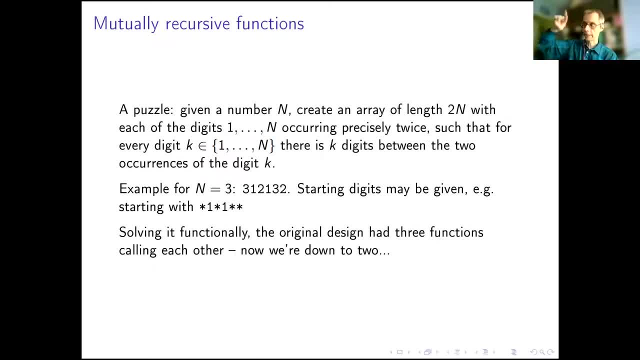 recursive functions in the first talk, because of recursion was the elegant engine of doing stuff and dividing problems into smaller problems and building a solution out of that, and we've- we've seen that several times. What you can also have is mutually recursive function. 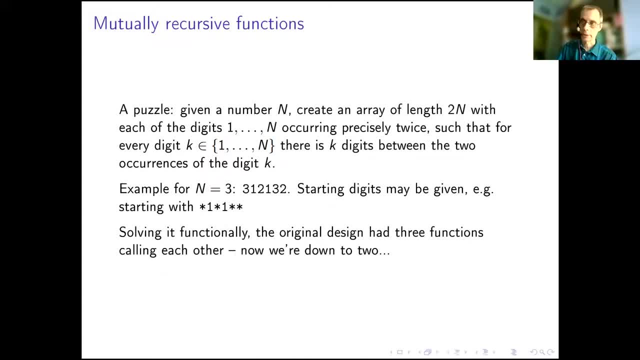 And I don't want to go into details, but I have an example with a source code that I will also put in github. And if you, like me, and you get a puzzle and you think actually it will be more fun to write a program that solves this puzzle than to solve the problem, the puzzle, myself, then 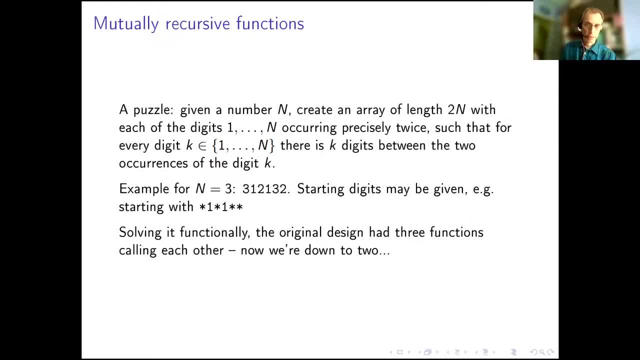 Then you will probably have done this before. So, As an example of a puzzle, you're given an numerical array of length To end and you want to place the digits one to end into it so that every digit has every did it? K has K digits. 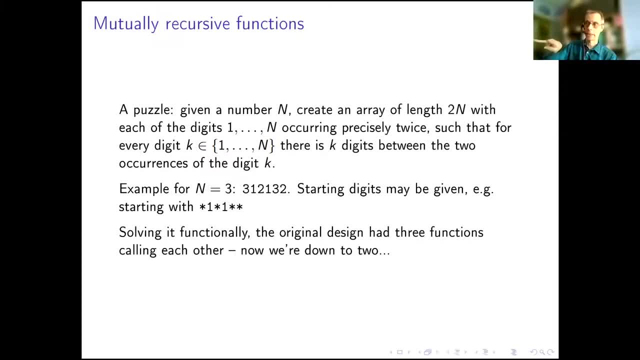 Between the two occurrences of the digit K, if that makes sense. so between the five, if there is a five, you have five digits. between the two fives you have four digits. between the two force, you have one digit between the two ones, and every digit occurs twice. 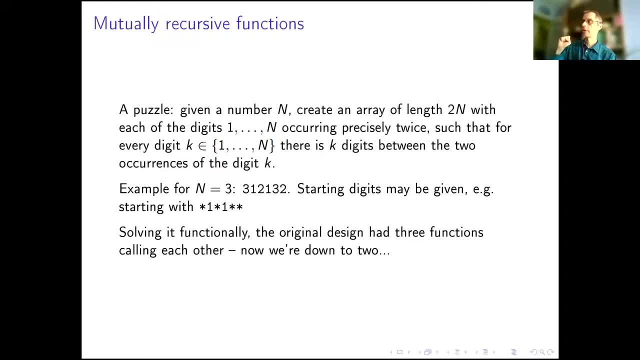 So you want to have a function or something that solves that problem for you, Given initial constraints- the size of the problem, perhaps, And so here's a short example: if industry then you want to have, maybe you're just given the ones- 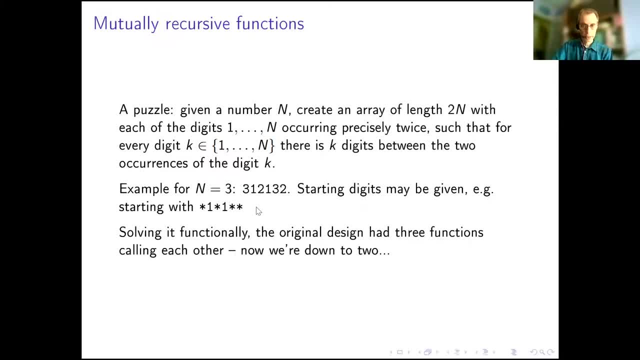 And you want to try and find all the solutions, or at least one solution, and it will put. you can see, this is a solution. between the three steps, one to one, between the twos you have one or three, and between one. is this just a digital? so that's the solution to this problem. 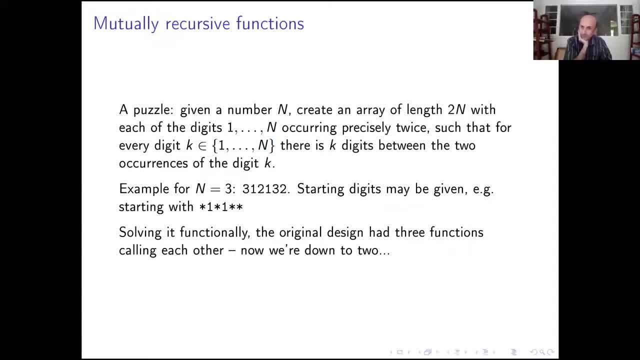 Now, Sorry, Is there always a solution? there's not necessarily always a solution. yeah, it depends on the starting, or there may be more than one solution. it depends on the starting conditions, Thanks, So originally, when I designed this, this solution, I had three functions mutually calling each other. 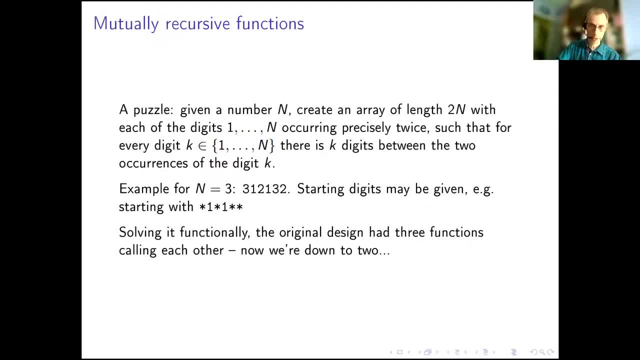 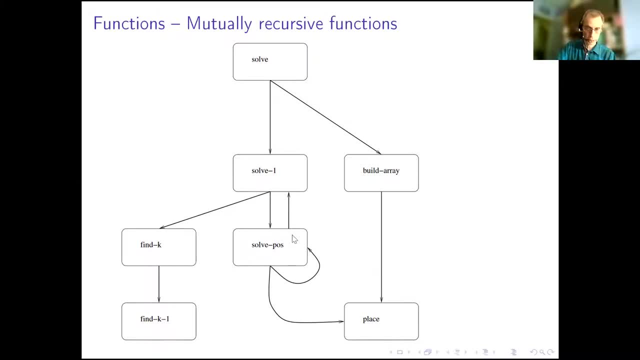 I think in the revision it's just two functions mutually calling each other, but the call graph looks like this: So there's a Top end solver and it calls the various subordinate functions and then there's a recursive engine inside of it that will actually do the solutions and 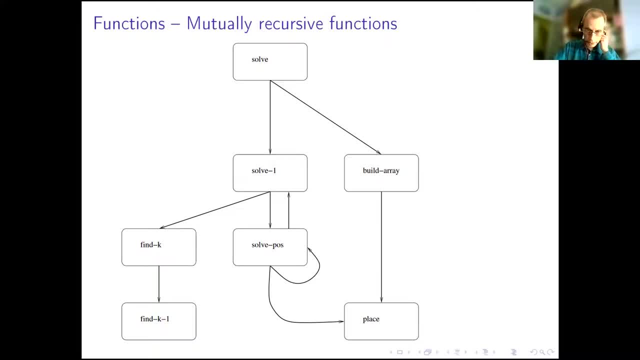 I don't want to go into this detail here, in details here, because but I will give you the source code so you can go through it at your leisure and and try and find find out how it works. the thing to point out, though, is if I use spcl, which is my normal. 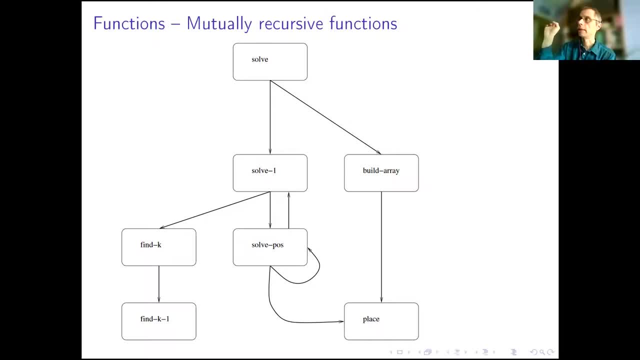 Common list implementation. it will complain if I write a function that has That tries to call something That hasn't yet been defined, And that's because spcl compiles things as soon as it reads them. Now it's still Okay, as we saw last time in the last talk. it's okay for me to have parts of my function that are not defined. I just get a warning when I load them. but it will still run, provided that the thing that i'm trying to call 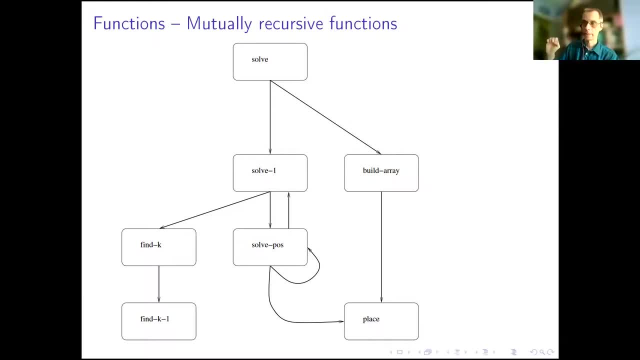 That everything I try to call has been defined, or if i'm capturing an undefined function exception or something. So it's okay for me to have parts of my functions that haven't been defined yet, but I still get the warning when I load them. however, if you do your things in labels, 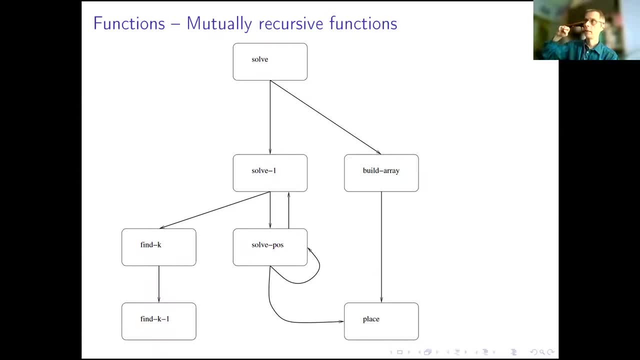 As your room. if you remember, labels introduced the Locally defined functions that could be cursing call themselves. they can also call it Other without any warning, because it sort of creates a little space around the functions that says i'm enabling the functions that I defined locally to call themselves, but they can also call each other. 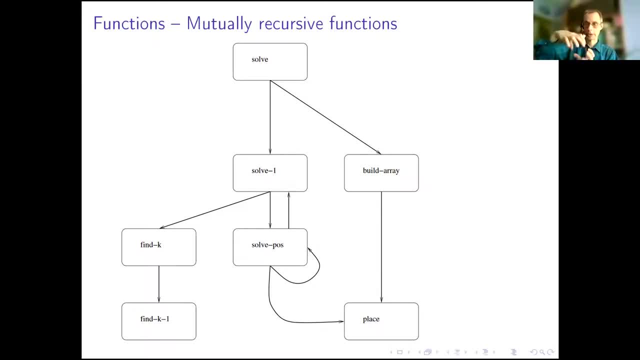 So if you're really a purist and you want to say, well, these, these functions, call each other and they needed each other to be defined together, you may choose to stick them into a labels construction and then just say that yeah, these are now together and they call each other. 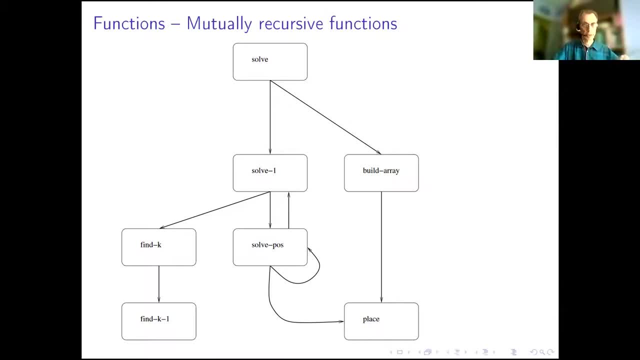 So that's just an add on to the discussion we had last time when we talked about what the when you should do labels and when you should do standalone functions. it's a little bit of out of taste, but if you want to emphasize that functions can call themselves and each other, it may make sense to stick them into labels. I think in this particular problem I have done both, so you can see what they both look like. 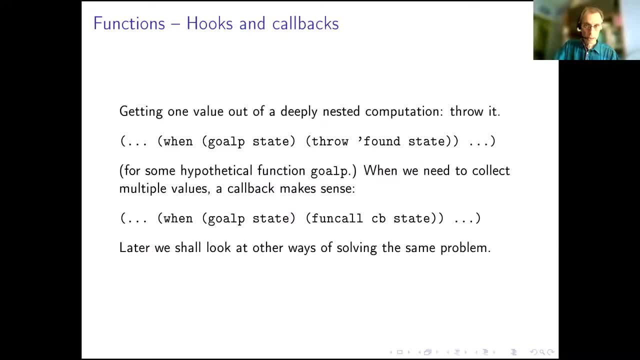 Okay, moving on. So I wanted to talk a little bit about how we use functions in practice From various Things. so if you imagine that puzzle I had before with the ones and threes and twos and stuff, now it may be that there's more than one solution and I want to find all of them. 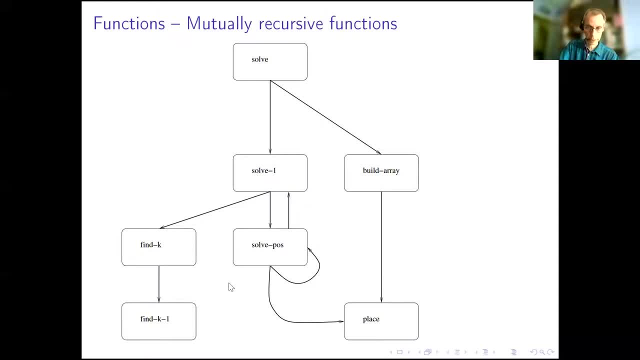 But inside of this call graph it might have gone really deep into it and there will be a stack that I need to keep. there will be State and and lots of things that I need to keep track of, so I don't want to throw that away if I want to find all the solutions. 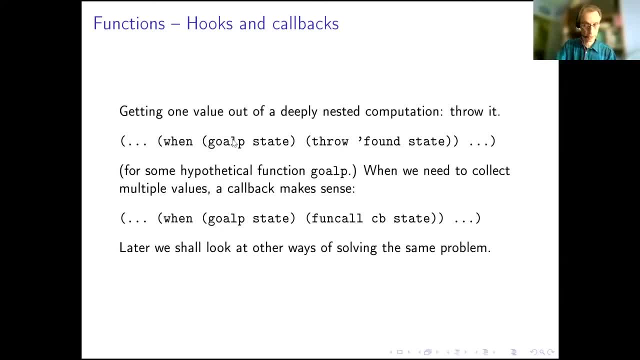 If I just want to find a single solution, it's Okay for me to just say: if this is a goal state By some hypothetical goal P function, then I just throw found and then say what the state is. so this is just my solution. but if I want to keep going and find all solutions, I would probably want to be able to get back to it. 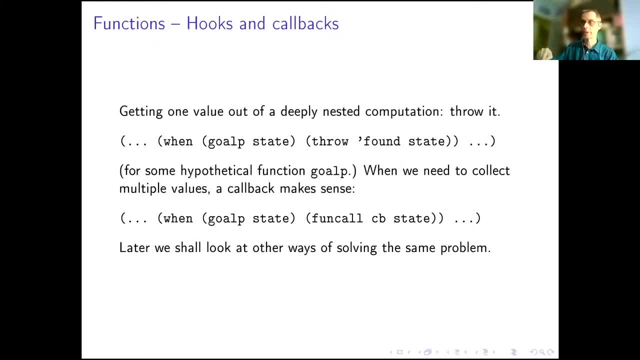 So the we should see later somewhat more advanced methods for doing that. but one option is to pass a call back into a function that says: Whenever you find a solution, then call this call back on that solution and then carry on working And that call back printed out, it could save it to a file, it could gather it into a list, it could do sort of whatever is I wanted to do, and that is just a useful way for me to get things to, to accumulate, while eventually the function will unwind itself as it goes back up the stack here and say I have found 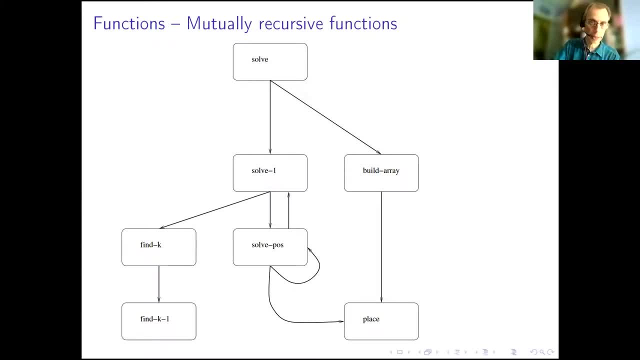 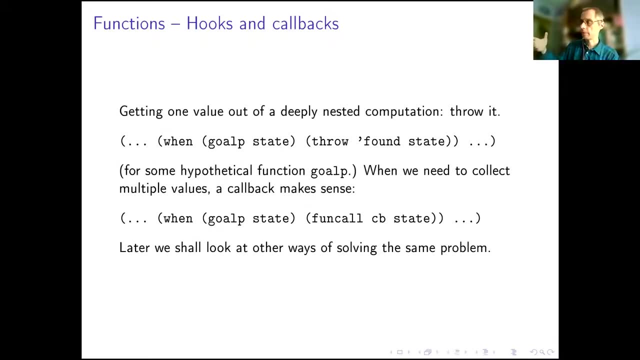 Now find all the solutions because it's a finite search space. So that's just a way of saying you can use functions. because we can use functions as arguments, I can pass a call back into the My big solver function and every time it finds a solution it will call that call back and the callback will then do something sensible with it. 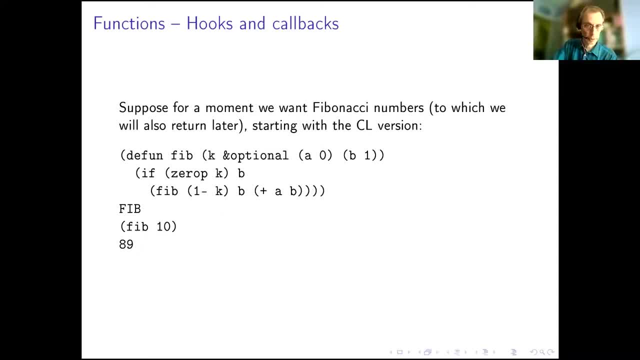 So let's suppose for a moment we wanted a Fibonacci number, And this is my common list implementation. It takes the nth number starting with zero that I am looking for, And then it takes optional parameters which actually passed in as my Initially. when I call the function. they're not used at all, but but then they get defined because I haven't specified them when I call it. 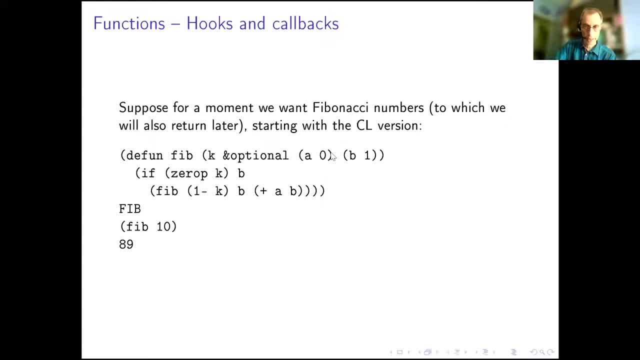 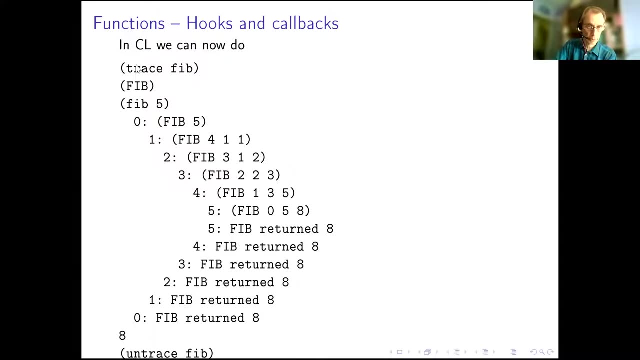 So when I say fib 10,, for example, then a, a just gets initialized to zero because initialized one, and then it will start calling itself and recurrence. And this is what it looks like. if I trace it then you can see that there's. I call the function the first. it says just fib. because I have traced the function. 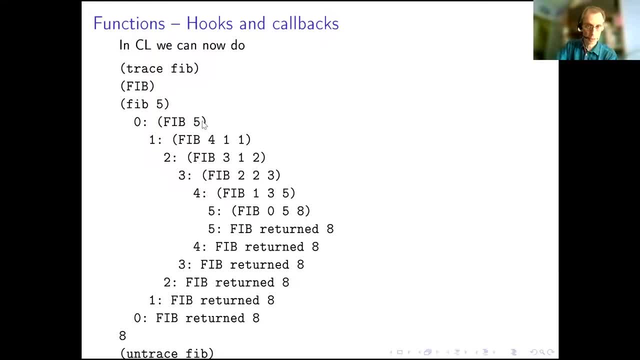 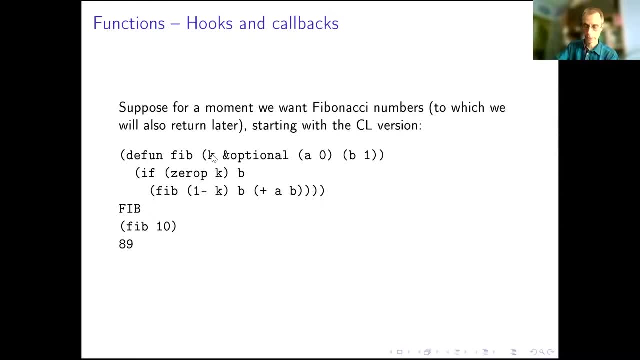 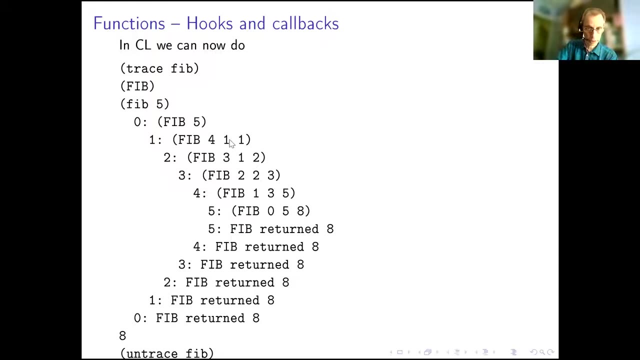 And then I call it with five and you can see what the call stack looks like. it says five, then it goes to 4321, zero, Because the first element, K, just just counts the number of numbers that I want to, or the nth number, and then you can see the remaining variables get set to 123. 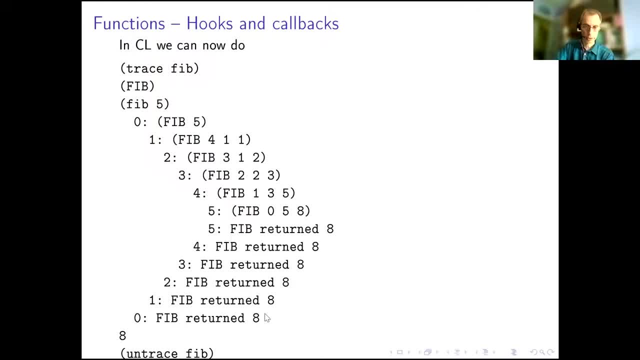 five and eight and eventually it just returns eight and goes back to the top and I can untrace my function after that trace obviously is is an extremely useful thing to have when you, When you're debugging functional programs, because it takes whatever comes into the function and it says here's what came into the function. then it looks at what comes out and says here's what came out and 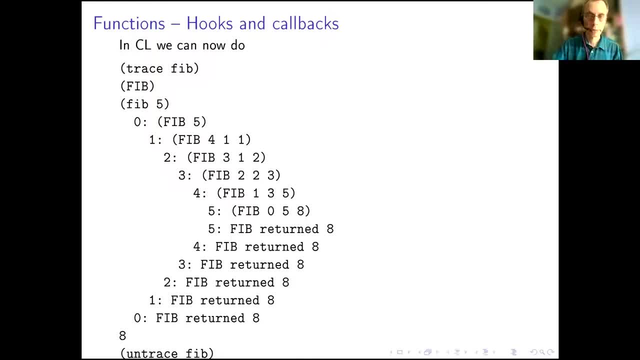 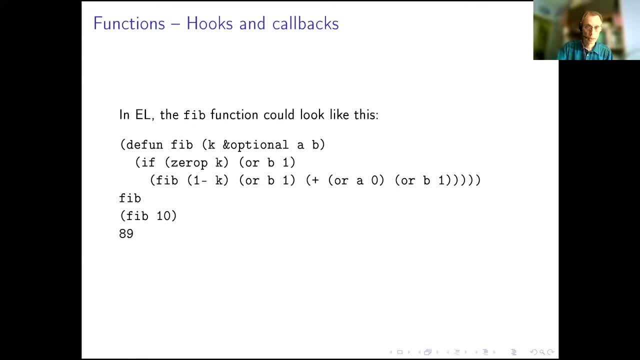 Then you can see whether the function actually behaves as you intended, And if it doesn't, then you can try to debug it. obviously the trouble is that this is common list and he max doesn't have trace. So suppose I wrote the same fibonacci function in emacs which looks like this. so he max doesn't have default values, as we saw last time for the optional parameters. so I use all be one to say if he has been defined, that USB, and if he has not been defined, then use one. 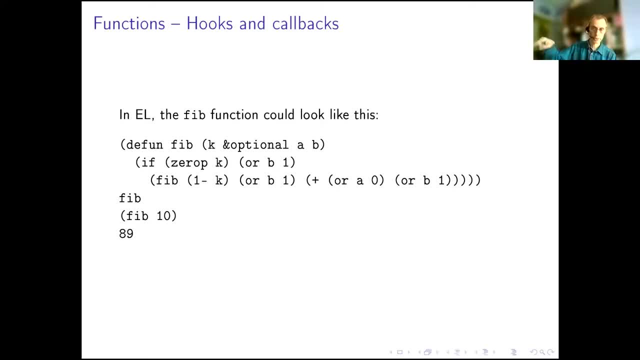 Obviously when it starts recursing. then be is defined, because i'm passing in the optional parameters, it's just in the very first call that it's not defined. So if I had spent more time on this and I could, I would probably have put in maybe a main function and a recursive functions inside with labels or something. so it became a little. it becomes a little bit tidier, but 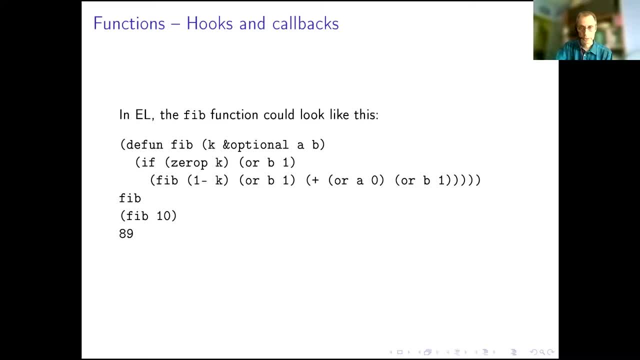 Who cares? So this function, as you can see, works exactly the same way. it does exactly the same call process, exactly The same parameters in. so on the in the recursion be gets passed in for the a value and a plus B gets passed in as to be value, and then it recurses. so okay, hits zero. 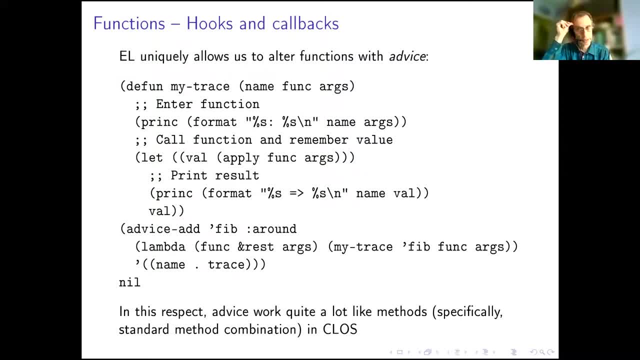 So in the max we can do something different, because he max has something called advice for functions. So suppose I write a function just to help a function called by trace, which takes a name and a function and it's arguments it prints, Formatted. 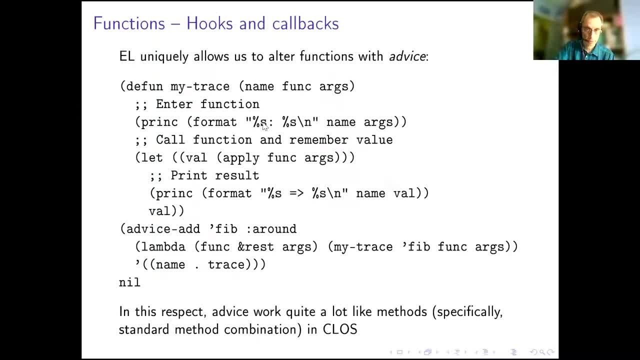 Strain of the name and the arguments. The name is just a simple, so it just helps me what function is being called, Because the function might just be a Lambda expression and not have a name, or it might be a closure. it more likely it's a closure in this case. 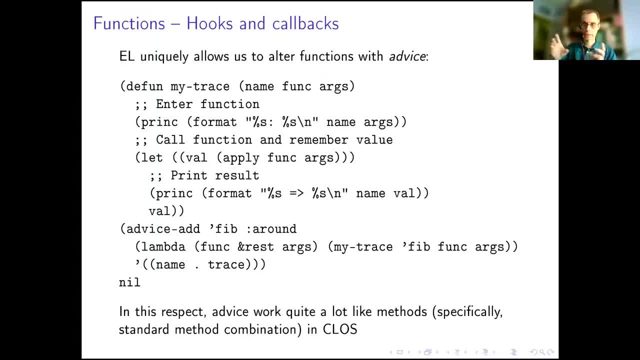 So it doesn't have a name. so the closure at least mean on the wiser. so I want to have a tag and name that says what it is that i'm i'm calling here. Then it calls the function using apply and it is saves the value in some. 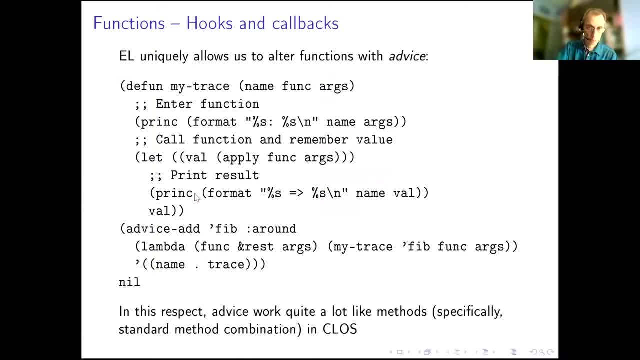 variable says this is the value, then it prints out what the value was and finally returns the value. so the effect of using my trace is that It, If you like, intercepts to function call and says your function. you're about to call a function with these arguments. then it calls the function and after the function has been called, it says this is what the function returned. 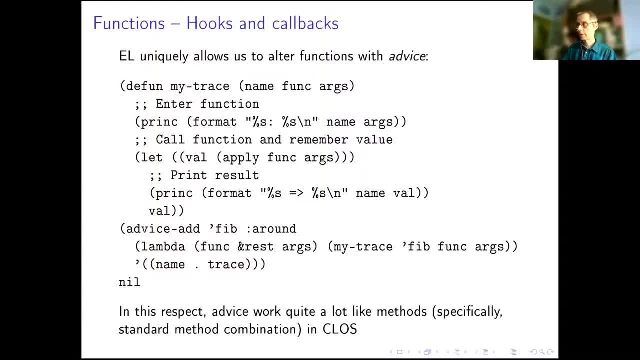 Assuming the function returns something, If the function runs forever, if the function raises an exception, then this, this argument will fail. but we can always make more sophisticated if you like and to to at least catch exceptions and stuff. anyway, In emacs you can add advice around a function. so what I tell it is the simple: fib names my function and I want to write: add an around. 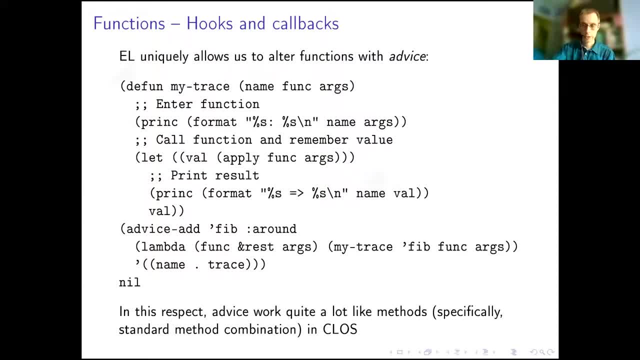 method and around advice to the function And all it does is to carry the My trace by finding my name in the function call and then it passes in the function and the arguments. So advice is a little bit like intercepting your function call. 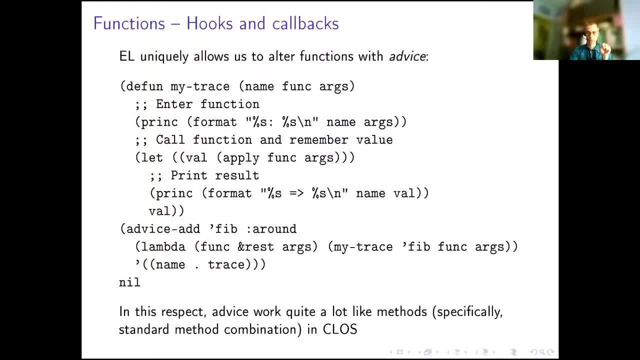 And you can tell. you can tell emacs when you want to intercept it. so if you look at this keyword parameter, call on around, which is a keyword It says I want to accept, I want to intercept the call and essentially not call the function at all. I want to call it myself in my trace function. 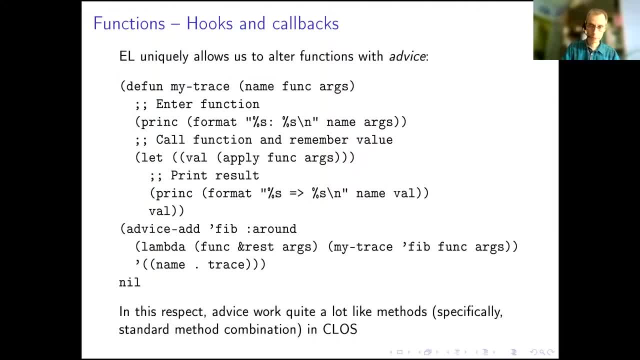 And I don't want emacs to call it at all. I could also add before or after, with before the advice will run, before the function is called, with after the advice is run, after the function is called. or I could add both before and after methods and. 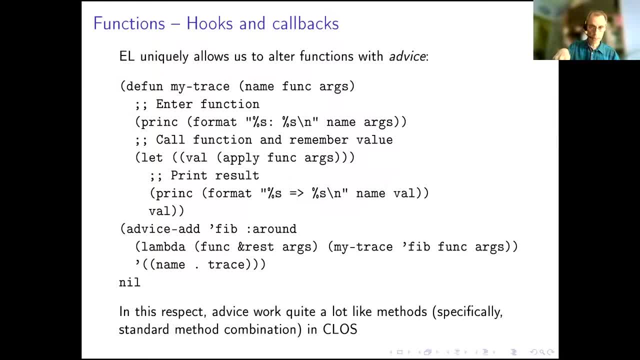 And then, of course, before will be called before the function and after the after the function. So, as you can see, i've also given it a name using an, a list, And there are only two values that are accepted to. parameters have accepted inside the a list: the name and. 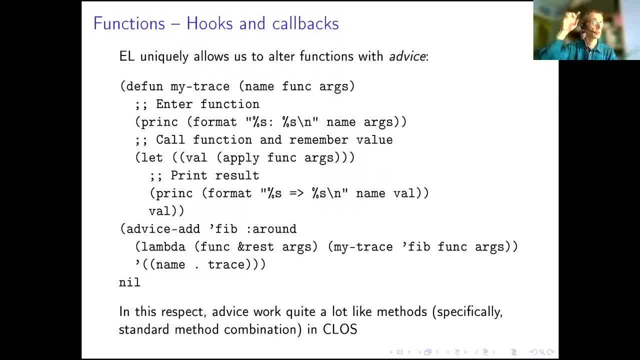 Something else- I can't remember what it's called, but it's- it's said to- to add the in which order, which priority you want to give it, Because they could be other around methods to this fib function that somebody else's put there, so I might want to say whether my around method should run first or or or next. 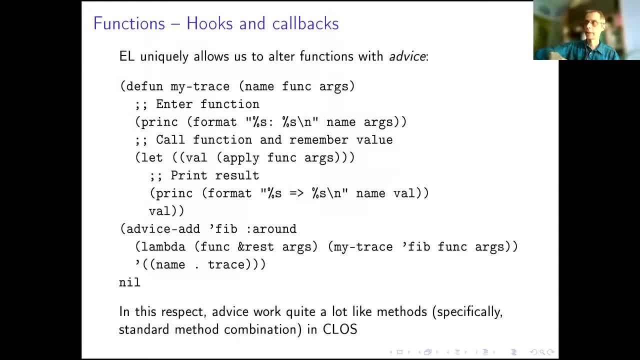 And I call it an around method. this is not what emacs calls it, and I call it an around method because see loss, the common, this object system calls it an around method. so I can't help call it an around method, but but emacs calls it an advice. 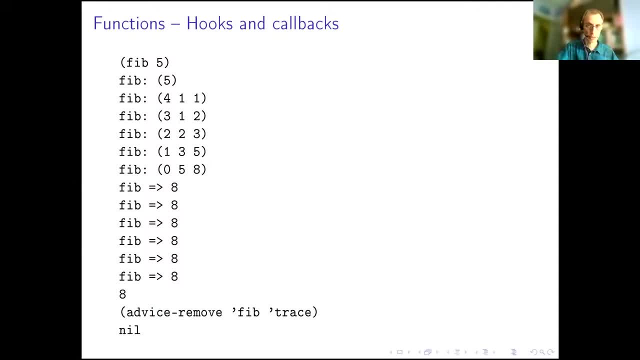 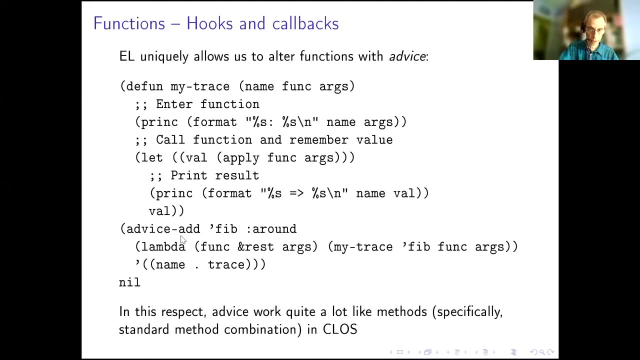 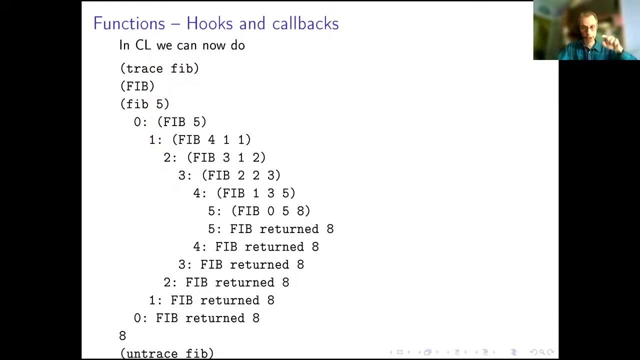 So this is what happens in the Once i've installed this, then I call fib and you can see it doesn't quite have the Nice formatting, but I could introduce that if I worked a little bit harder. But it gives me exactly the same trace value of the function calls and it's exactly the same values that I had before. so you can see it says: returned eight because it's recursive call and it just says how often. obviously, every time it returns eight because the 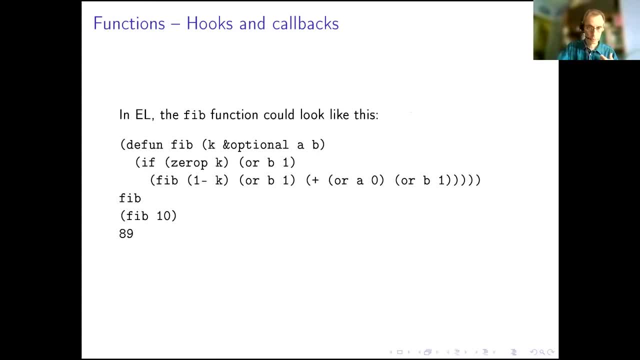 recursion is the last part of the call, So So I just end up getting this long stack of eight and it's just returned and eventually gets passed back into as the final value of the function, and then I can call advice, remove once i'm tired of tracing it and it will just take it. take it out again. 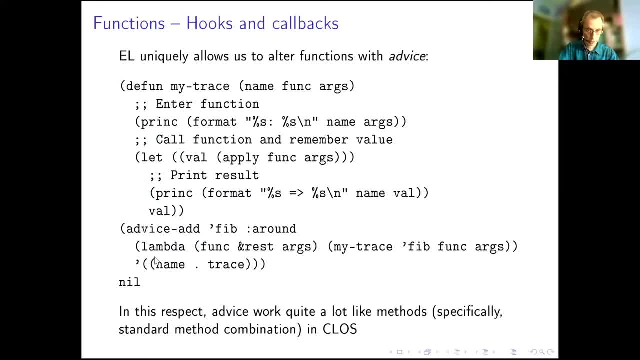 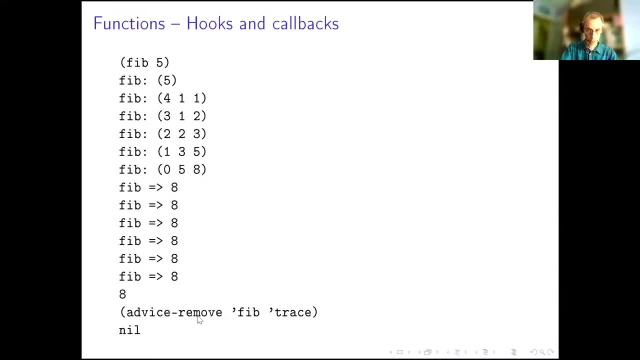 And here it's using the name that I gave it before. so here it says in my a list name trace, and so traces the name that i've given my advice. and when I now say advice, remove, trace, then It will look up for that, look for that name in a lists, like we saw in the last talk, and just remove it and then effectively the function is on traced. so this is sort of a cheap and cheerful way to build traces into the Max and debug your functions. 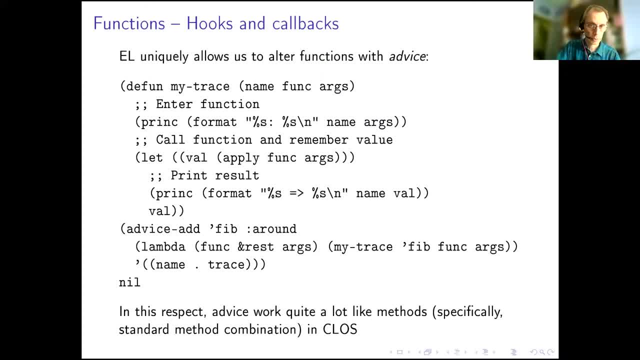 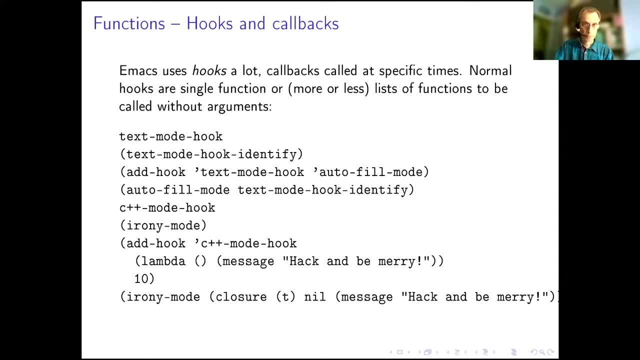 Which I think is pretty neat, Because for a long while I thought that he makes didn't really have traces at all. Right, He makes also, as i'm sure you've probably seen, if you've done anything, Any kind of 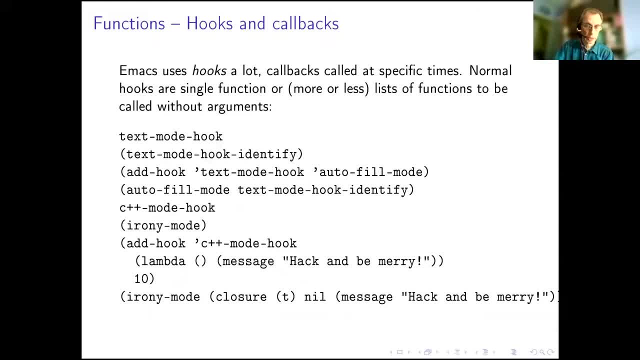 Emacs programming it will have lots of hooks for customizations. so there's a variable called textbook hook, for example, which will call contain some, some function or other, And you can add a hook to that. so for example, if you wanted to have auto film mode, you could put the, put it in into the text mode hook and every time the max enters text mode it will then also run also film mode. 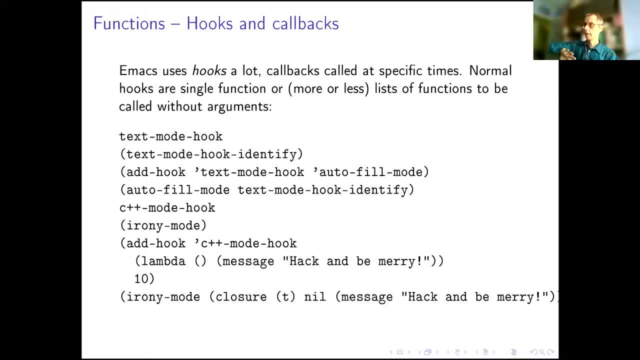 And so you get also film mode every time you run, Every time you're in text mode, And that's probably better ways of doing that. but it's just. it just illustrates how you can use the hook to customize the Max, and there are lots of folks for all kinds of things. 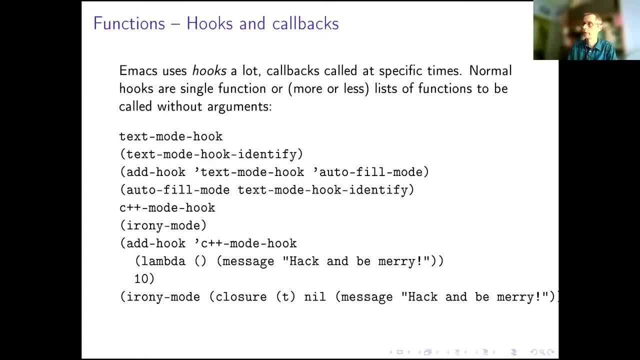 In X in fact talks about two kinds of hooks: normal hooks and abnormal hooks. And normal hooks can be either a list of functions that get called with no arguments, or There are also Supposedly functions and just just a single function. so not a list of functions, but just a single function. 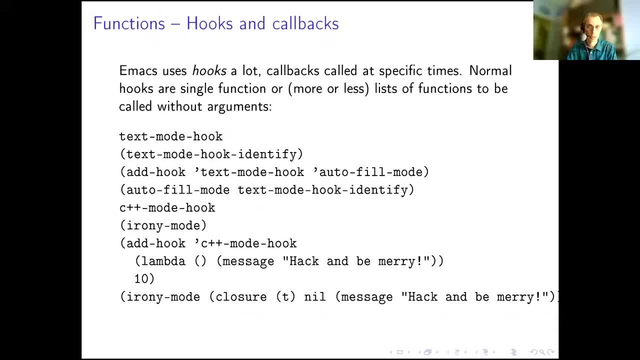 So I can't actually think of any at the moment. The normal hooks I can think of will have a list of functions to call when their event triggers. So here's another example: if I evaluate C plus plus my hook in my Emacs, I get RNA mode because for some somewhere, 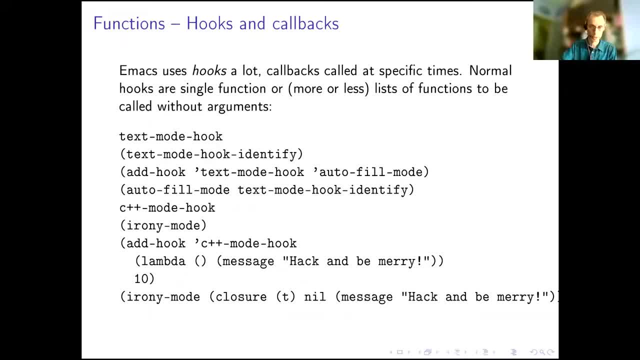 Inside my Configuration something has added RNA mode into my C plus plus mode hook And if I then add another hook, which is just a Lambda function that says a message how can be merry? then every time I go into C plus plus mode it will switch into RNA mode and it will give me a nice message that says: how can be merry? 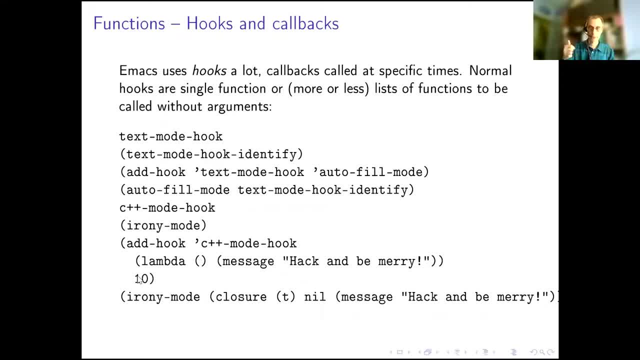 The 10 is a priority. that it where I want to put it. so can be a negative number or positive number and the hook will put it in according to the Priority you give it. So you can see the hook is actually returned by a hook. so you will have irony mode there and it'll have the closure of my my message thing. if I gave it minus 10,, for example, then the closure would come first and it will have iron RNA mode next. 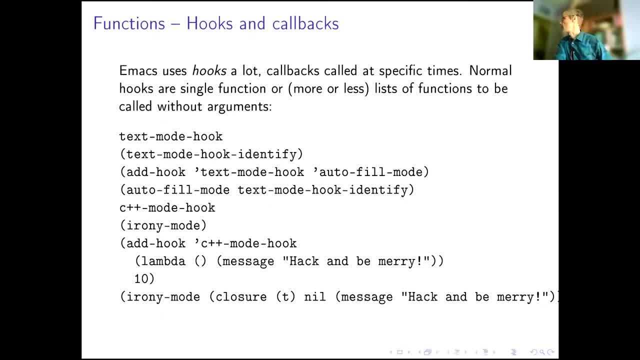 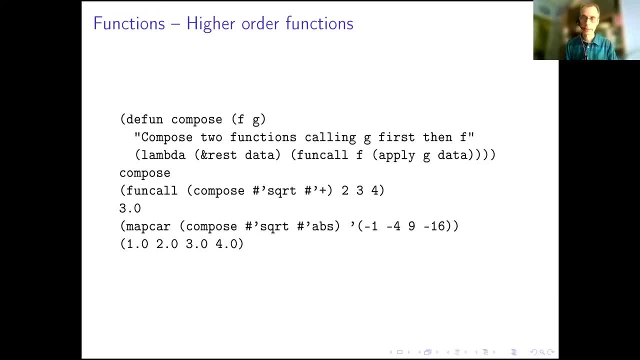 Okay, so that's it for the, for the hooks. I realized i'm sort of racking through topics a bit here because I wanted to get all the sort of loose ends Out of the out of the way before we get into the some of the more the larger topics. 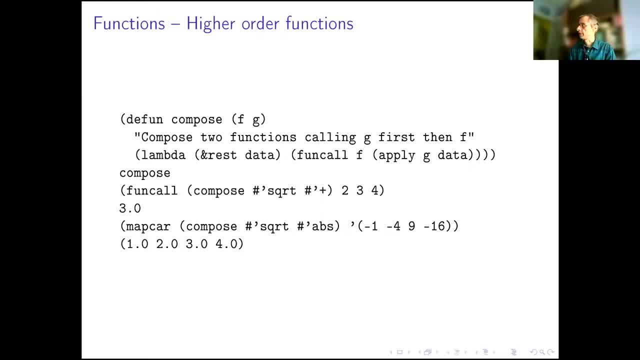 and I still think some of the loose ends I are useful, like this tracing thing, for example, can be quite useful because you can. you can put that tracing thing into a macro or something clever And it will then extract the symbol and use that, my trace call, to wrap around the actual function call. 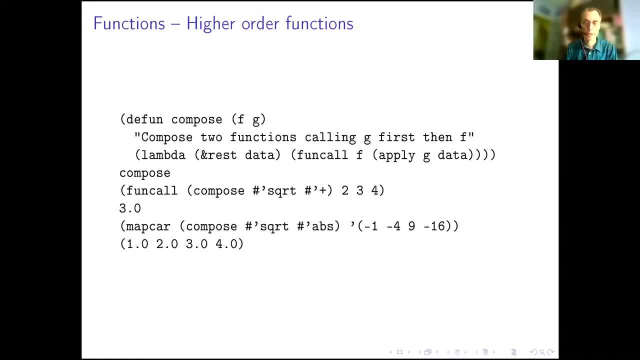 And it will then trace things for you and dump things out on your screen, so it can actually be quite useful instead. so this is a nice alternative to putting debugging statements into your function and re reloading them. So we talked a bit about high order functions when we talked about lambdas, and here's another example. compose is an example where you have a function F and G and you want to call G first in this case, and then F. 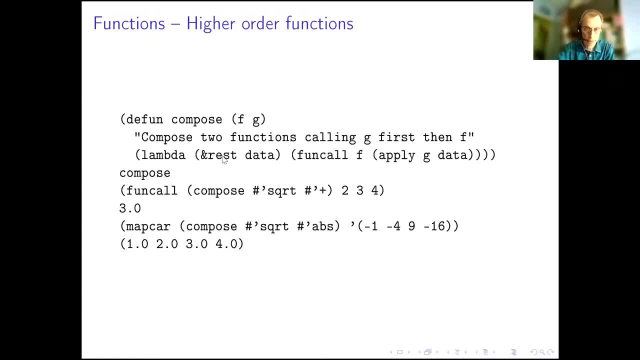 And this is Pretty straightforward: lambda- Take some data into it and then he calls G first on the data using apply, because data can can be a list of things, Because i've captured it with rest- and G then returns a single value, which I then used to pass into a function called F, which must take a single value. 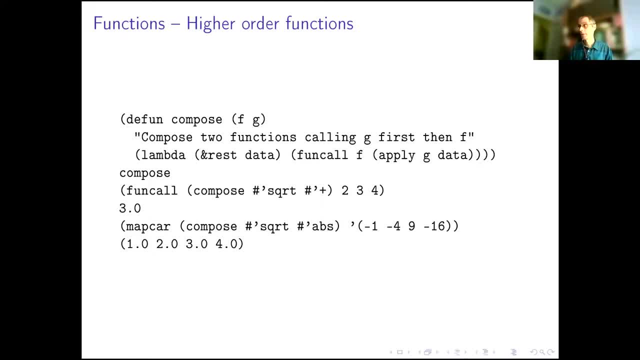 And even in common list. if G return multiple values, In the function call, still only the first of those values would be used. so it was in even in common list to compose function will look the same And you can see how it works. if I, if I type control, square root and and plus on a list, then the list gets wrapped into the data. the function G was is the plus, so it will sum the things together, which becomes a nine, and then we'll we'll take the square root of that. 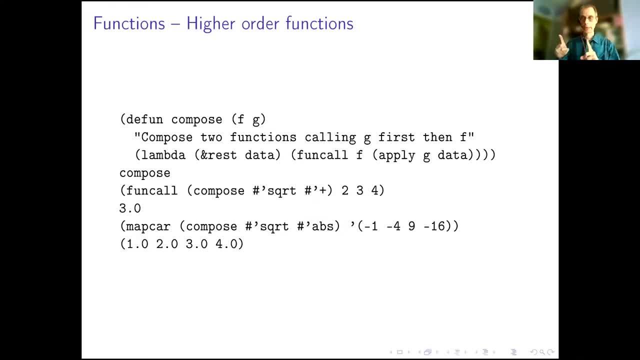 The differences, That the composition is created first, as you can see. so the compose function runs first and it creates a closure, the lambda which remembers that it's supposed to call G first and then F and then the. that lambda is called on two, three and four. 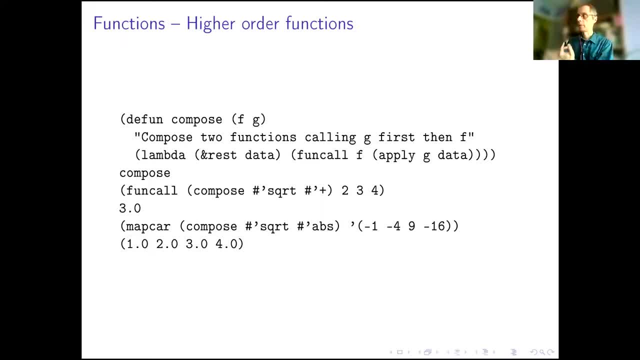 So the function has been composed before I call the first function. So that's why we work with higher order functions, why we say that I guess a function that takes functions as an argument, it returns another function which I can then call. So another example: compose square root and absolute value. so that gives me a function expressed as a lambda closure. 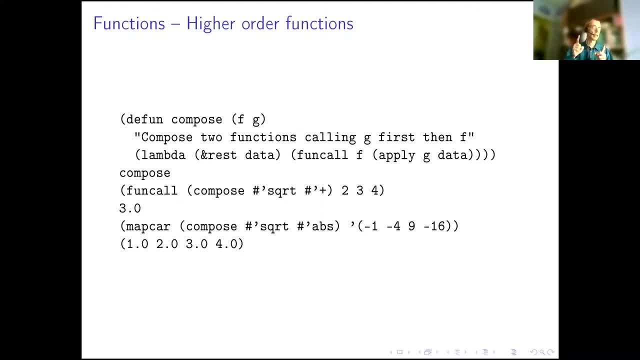 Which will take a number, and it will then take the absolute value 10 square root, And you can see, it has done precisely that Here: minus one, minus four, and it gives me one and two. So so the thing to take away from this is that we actually acting on the functions as arguments and returning functions which we can then call. so the function compose, if you like, is a function of functions. 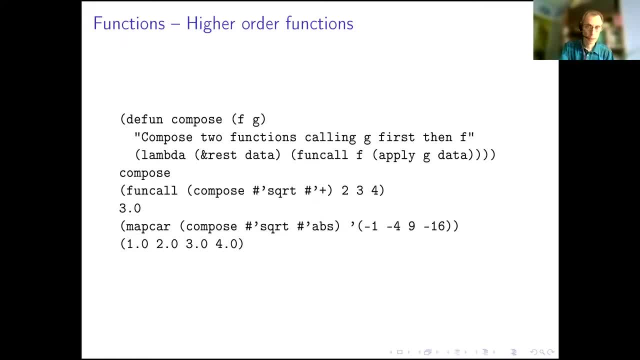 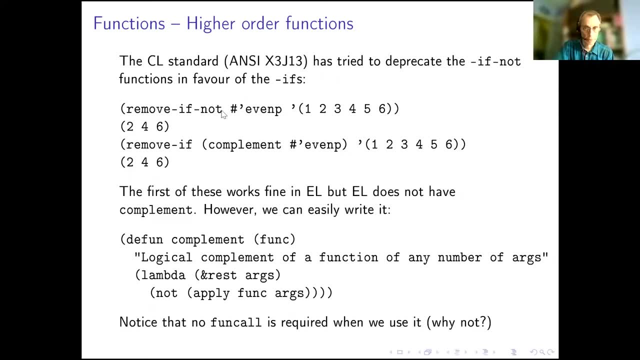 Because it's designed to be applied to a function. here's another common example: remove, remove if not. Is a common list function in emacs list or in common list as well, obviously. and so I can say remove if not even P, so remove a number if it's not even. 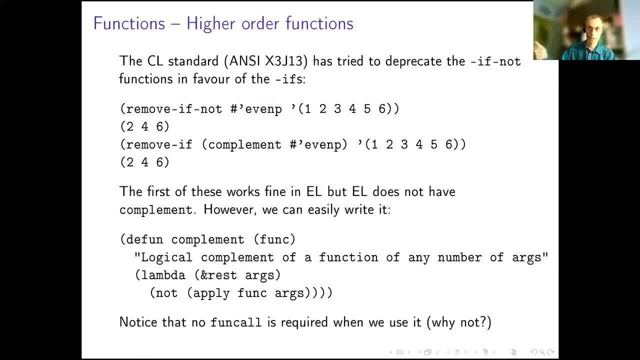 Which is actually a nice function to have because, as you can see, it essentially says select. if give me all the variables out of this list that are even numbers. Now, for some reason they have tried to deprecate that in the standards committee. 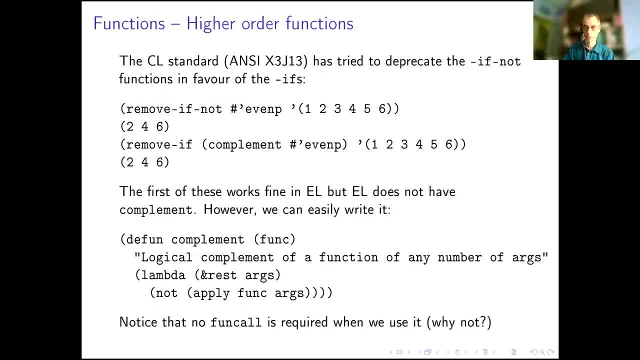 And saying you don't need remove if not, if you just have remove if. and it will be nicer to just have remove if rather than remove if not. I sort of disagree because I like remove if not as the concept of select if. But you could say: remove if, compliment even P, even as a predicate, and if I compliment it then obviously I get odd P. but if I wanted to express not even rather than odd, then 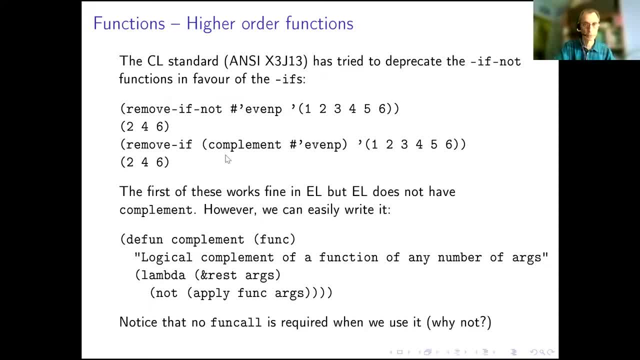 Like if it was more something, some more sophisticated predicate, then remove. if compliment predicate should express the same as remove. if not, Of course, functionally it returns exactly the same. but you also telling the programmer who reads this- which could be yourself- what you're trying to say. 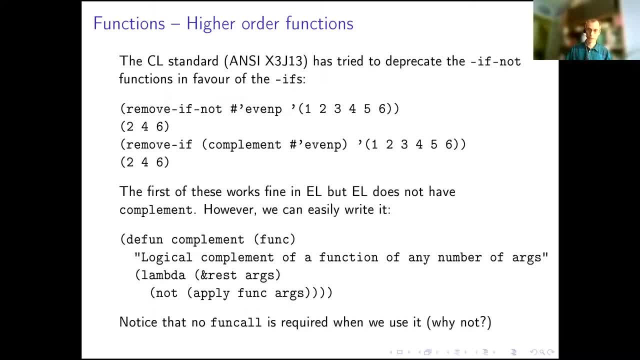 So remove if not could be expressing selective, or it could be Saying: remove every number. that is not even or something. emacs does not have compliment, but we can easily write it because It just takes a function and as a widget, which is assumed to be a predicate, and it gets the value that comes out of that. so it just takes the arguments- which could be any number of arguments- applies the function to it and then takes: not have that value, assuming that it's a generalized boolean. 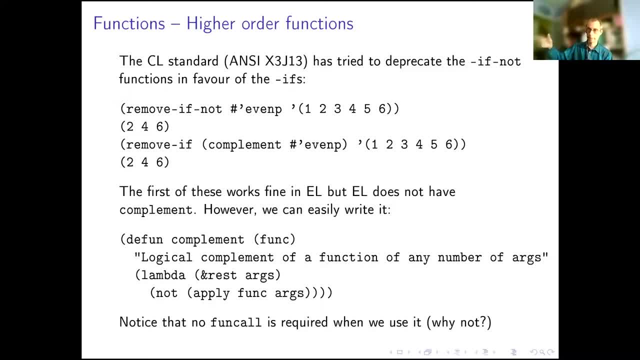 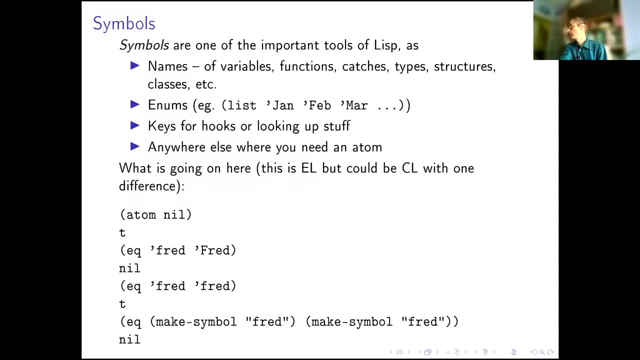 And again, what happens here is function is a function, and compliment takes is a function of a function, which returns a function that we can then call later, As You know, as any normal function that we have elsewhere. Okay, so that's it for higher order functions, and now we're getting to some of the slightly larger topics, and this is actually the last topic that I intended to cover today, but we can move on a bit if it turns out we have more time. 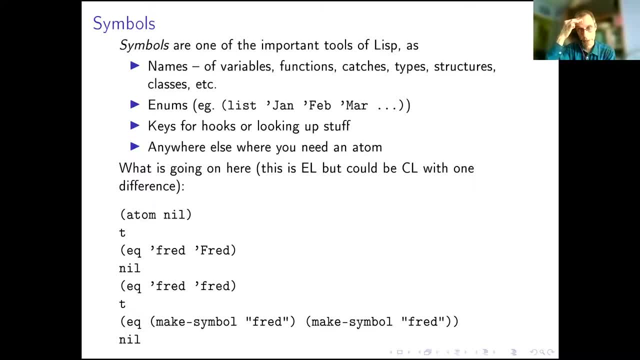 So I wanted to spend a bit of time looking at symbols as well, because symbols are quite powerful tools in list that you don't really find the equivalent of Those in in other languages. you find sort of Things like enums in in C or 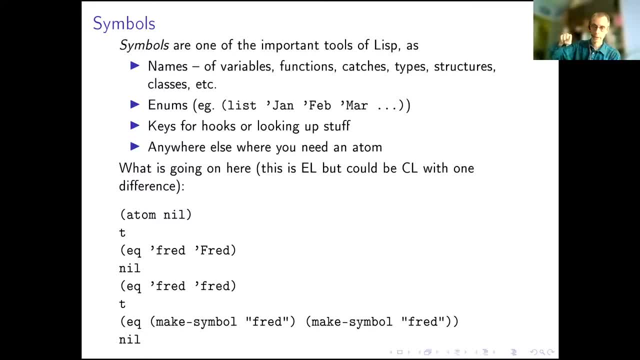 Maybe it uses strings in other languages, but, as we saw with the months last time, you can actually use symbols as very efficient tags for looking up stuff in a lists. we could use symbols as keys and and they can actually be used for for lots of useful things. so I thought it was probably worth looking a little more closely. 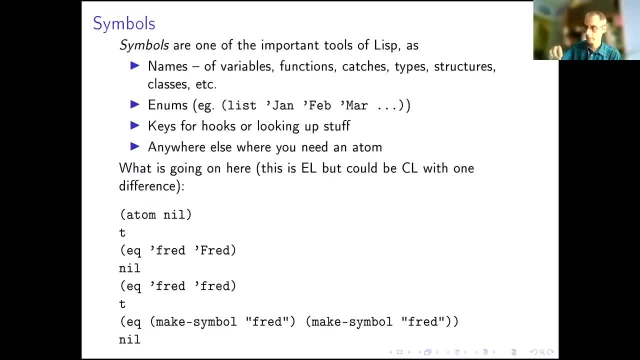 At what symbols can do, because they can. they can be sort of abstractions like enums, they can be names that can bind variables or functions or various other things, can name types And they can be keys and generally anywhere you need something that's atomic, something that is not a cons or a sequence. 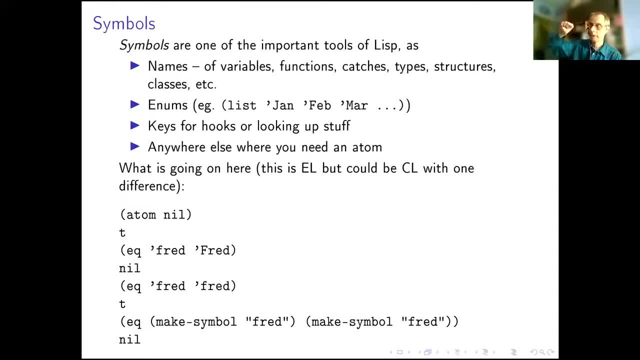 You can use it in principle. you can use a simple- and we've even seen that with the bindings, that you can bind them and then you can shadow the binding, like in the Lambda, with the letter inside it. you had the V that was bound to a value and then it was bound inside of that again. the V is still the same, simple. 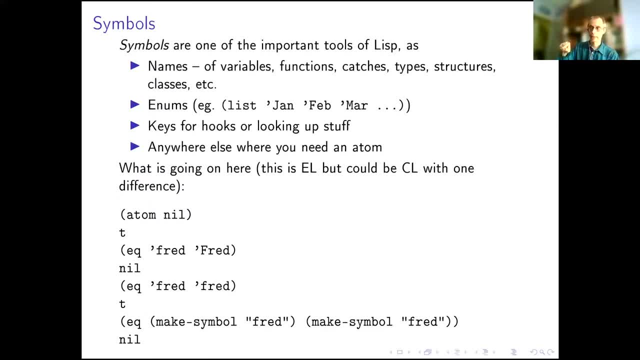 But depending on the context, we look up a different binding and will- in a later section we'll look a little more closely at that and how that can be really useful. So let's first look at symbols and see how far we get This. 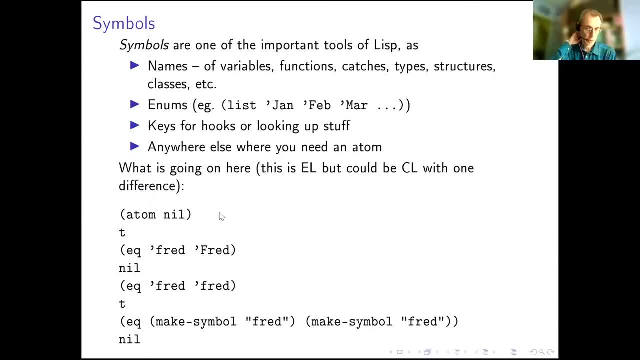 middle is a symbol and it evaluates to itself. and then I asked whether middle is an atom. and it is, because no, it's not accounts. mail maybe an empty list, but it's not accounts. so it is indivisible and it's. it is indeed an atom. if I say EQ, quote Fred, and quote Fred with uppercase F, then they're not the same symbol in emacs. 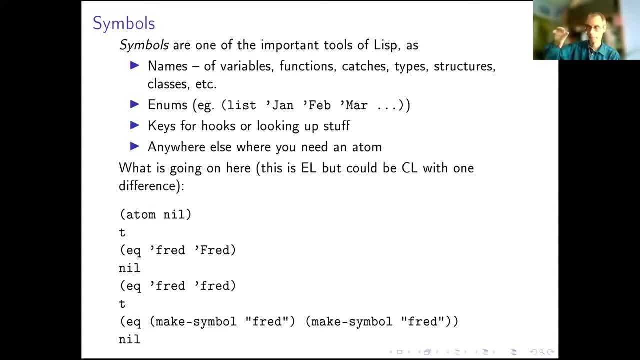 Because They have different, different symbols, because they have different, you know, capital letters and stuff. If I say, if you Fred, Fred, then I get T because he's true, because they have the same symbol. And if I say EQ, make simple Fred, make simple Fred. so I create two distinct symbols with the name Fred, but they're not the same symbol. so what's going on? 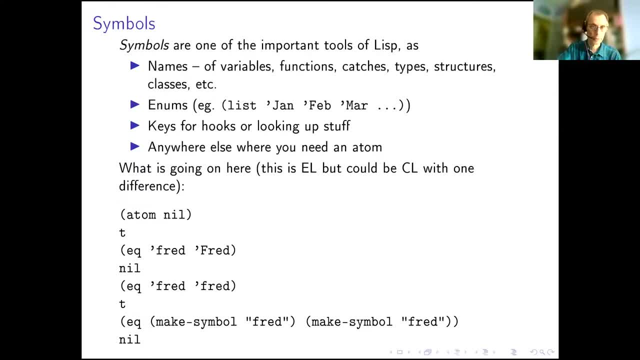 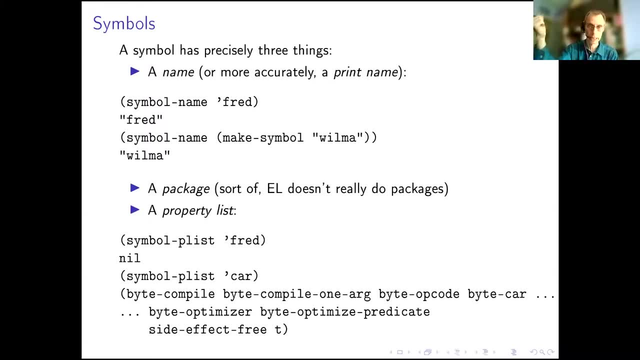 So let's look at what symbols actually do and how they're useful. A symbol has precisely three things in list. it has a name or, more accurately, it has a print name, which is the name that gets printed when, when the printer tries to print a symbol. 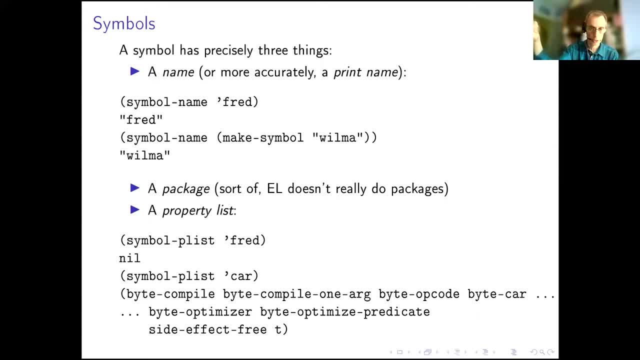 And it has a package and it has a property list And we'll look at those in turn. the name is: you can extract the name from a symbol by by using the function symbol name and it returns the symbols name as a string. So the string itself is a representation of the name of the symbol. the simple itself is not. 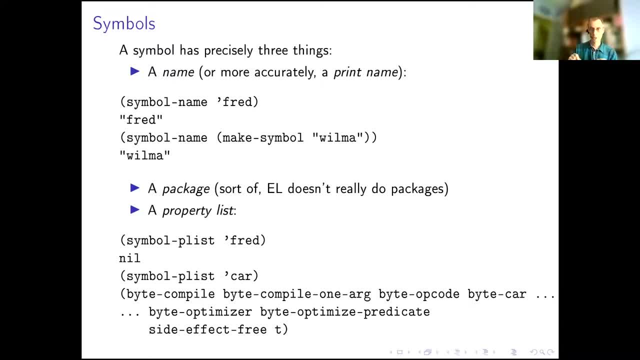 Composed of characters in any way. But once you've extracted the symbol name, then you have a string which is composed of characters. So it's important to remember that the symbol is indivisible, it's atomic, it does not decompose into fred or anything. 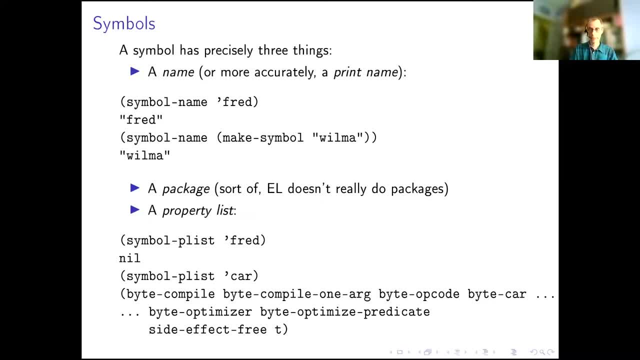 At all. it is simply a simple thread that is indivisible and untouchable. Conversely, you can create a symbol that, like Wilma here, and with a particular string, a particular print name as a particular string, as its print name, And when you then extract a simple name, when you extract the printing from it, you get the string back. it may not be the same string but it's got. it will be an equal string to the one you put in. 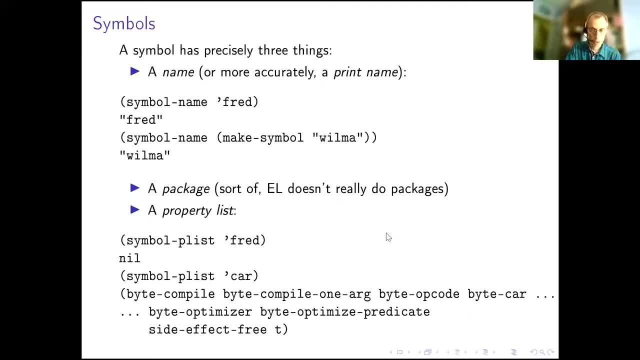 The package. i'll talk a little bit about packages, but he makes, doesn't really do packages, so I don't. I don't want to say a lot about it. and then it's the property list. the property list is an ancient piece of. 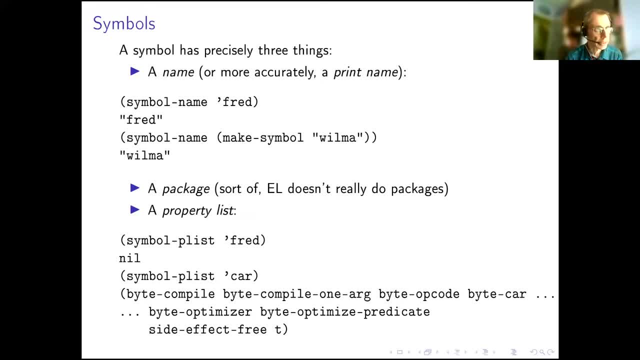 list technology That works a little bit like an- a list, in the sense that it has key value pairs, but it works in a slightly different way. there are some different important differences between a listen and P lists, But P less important To know because they're used by emacs. 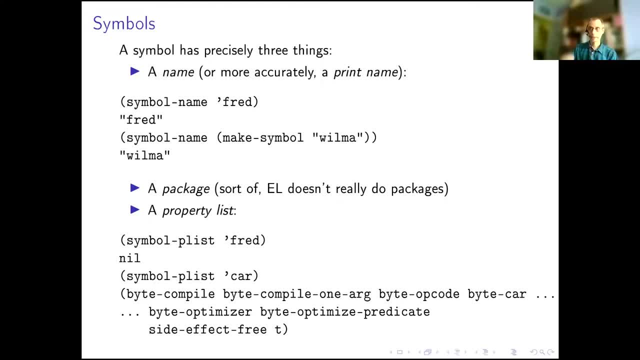 A lot In common list they're hardly ever used at all. I can't think of a single thing that actually uses them, unless you use them in your programs. But in emacs list they are used a lot here, for example- and just looked up the P list for for the symbol car, which, as you know, names a function- 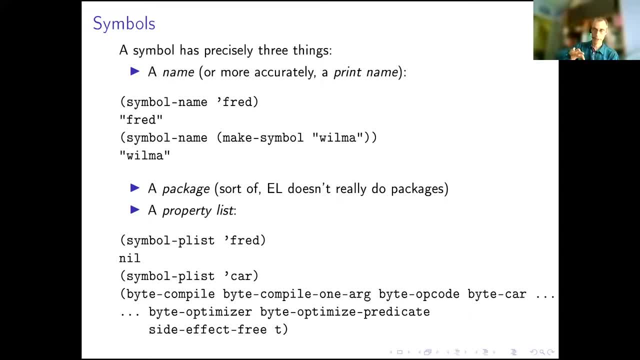 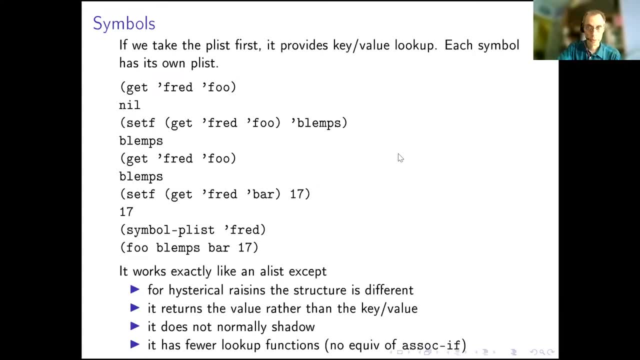 And it's. it will then have loads of stuff inside that explains to emacs and the programmer, if you like, Lots of things about how car works. So let's look at how P lists work in general and with a simple thread. I can ask what you know about the symbol food and it says no, because there's nothing in in the P list. 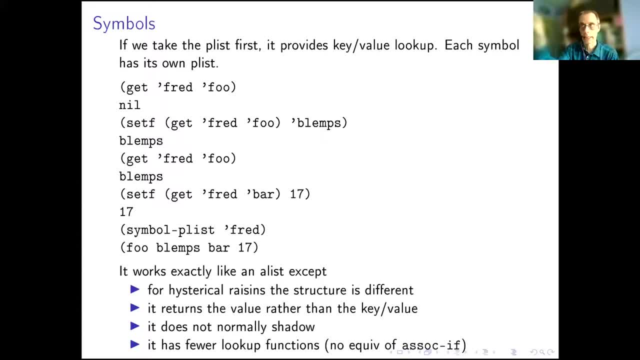 So the function get takes a symbol and a key and looks up that key in that symbols P list. So The The My simple here is Fred And my Key is food. and I look it up saying Is there's a value associated with food in the P list from Fred? and there's nothing. 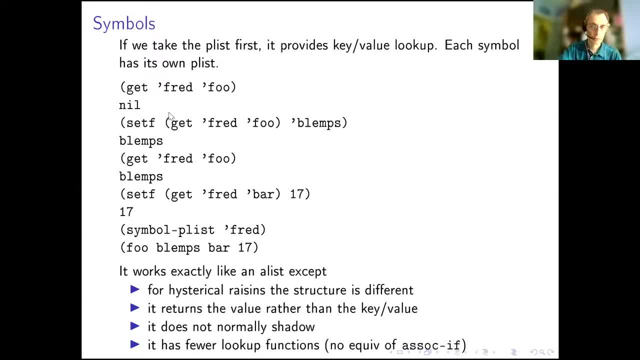 So it's important to get used to how these things work. if I want to set a value In fred's P list associated with a simple food, then I use the set function to set that place to a particular value and then I can use get Fred food afterwards and it will return precisely that value. 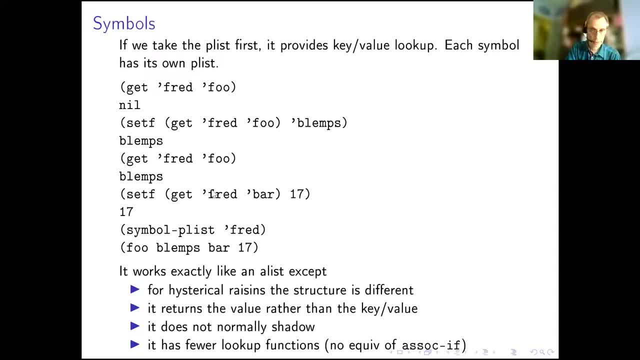 Because it's looked it up in the P list. If I then say get Fred bar, and I set that to to 17, so I then It sets that as well, and when I now say simple P list thread, you can see that foo. 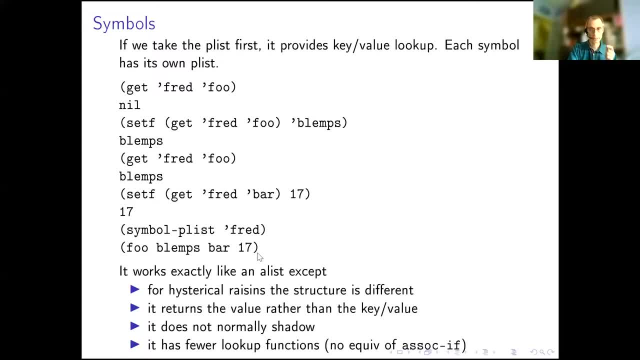 Has the value blimps and bar has the value 17.. So a P list is essentially, unlike the dotted path on, likely in that you saw an a list. they essentially key value, key value, key value. So a P list Always has even length. 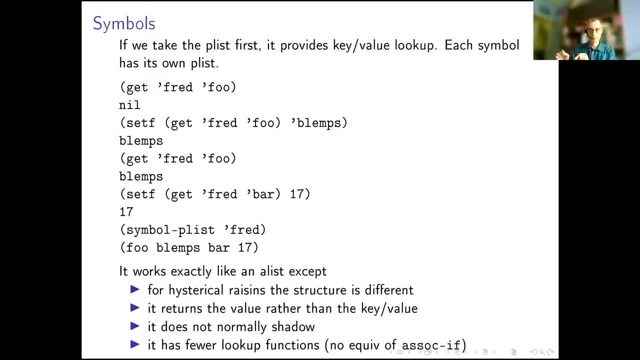 Because you always have a key and a value next to each other. And this is actually, if you remember, back to the last talk when I talked about I had just done some work and P lists and I was trying to show you how the ultimate a list looks like in any Max and I got confused because I was actually trying to look up keys using a playlist terminology. 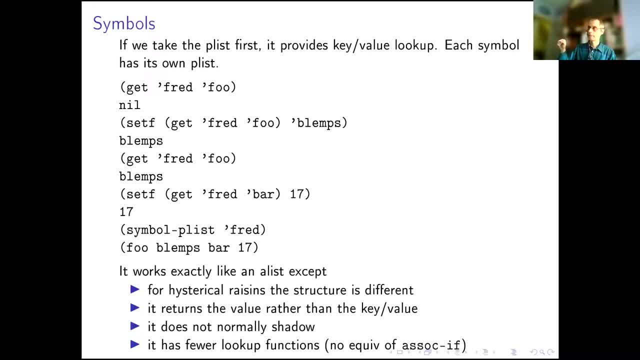 But I was actually also an. a list is an, a list, obviously, so it got completely messed up. P lists are used to store properties for a particular symbol. in this case, we just look at the symbol thread and we say what properties have so have been associated with that symbol. 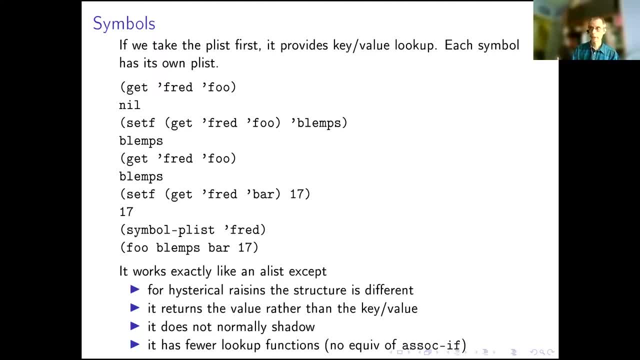 And those properties could be stored by myself as a programmer, or they could be stored As hints to the compiler, as he'll choose, to an optimizer or something. so they're just used by Either by the programmer or by emacs, or both. so I may want to check, before I said values in there, that emacs is not already using those values. 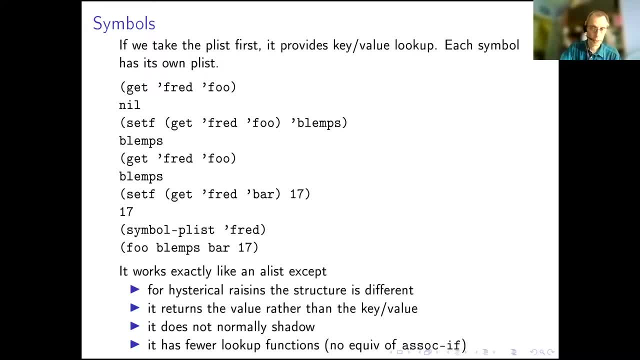 Now it is. P lists are less sophisticated than a lists because you can just do the look up you. if you remember the a list, it actually returned the console, which was really useful for lots of things. so you don't get that with P lists. you can still do the shattering if you'd like. 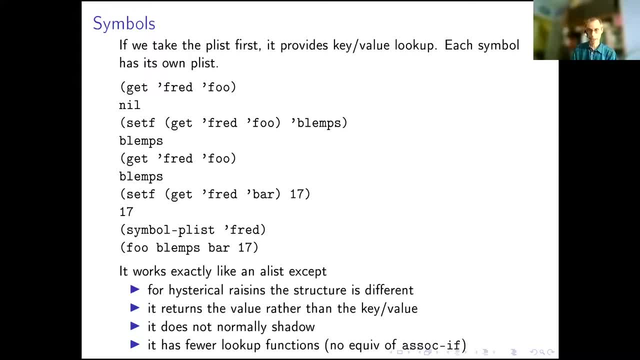 By pushing some for something onto the playlist. but Normally You don't actually do that because you would use the self to update the value of A property of a given symbol. So that will not do any shattering. it will just change that particular value if it's there and it will create it if it's not there. 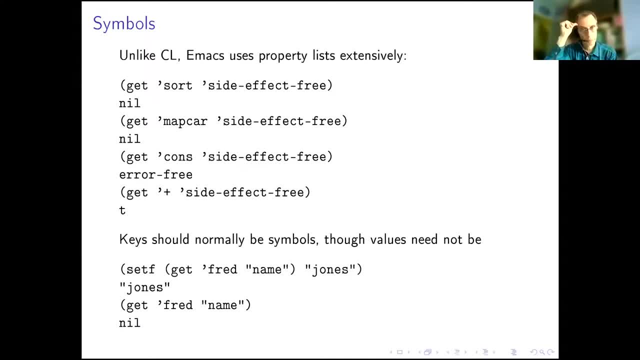 So emacs, as I say, uses them extensively so you can look up values like like sort as a function, The particular value that emacs likes to keep keep for these functions are stored for the symbol sort, Is it side effect free? it is not. his map car side effect free? it's not. if you look up car it will be side effect free. 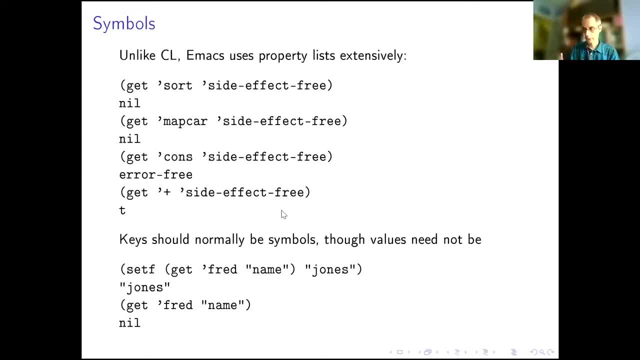 and So you get all of these product properties, which is probably have less interest to yourselves as programmers, but they are of interest to emacs when it tries to compile and optimize code. And also, you probably want to use symbols and not strings because, as you can see my on the bottom of the page if I try to set a key. 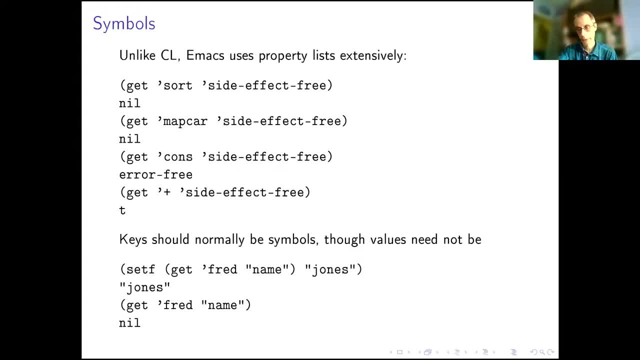 Which is a string, then look up will fail because it will use eql as the comparison function, so so that's not going to work. So all of this is just to say that the playlist exists and ordinarily you will not need to use that as a as a programmer, unless you really wanted to store stuff. 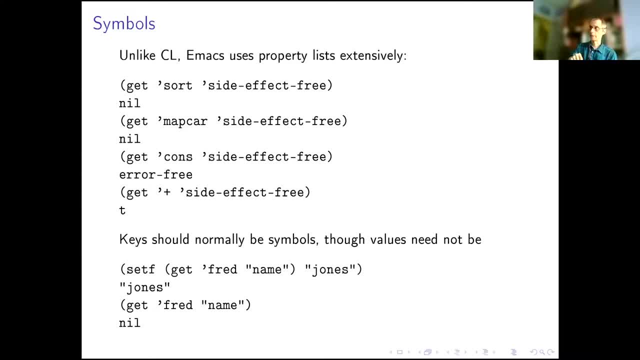 Properties associated with a simple. so the advice that I put in before on my fib function actually gets added to the fib symbols playlist In some format that makes sense, to emacs, and then when I say advice remove, it gets taken out of the playlist again and you know you can forget about it. 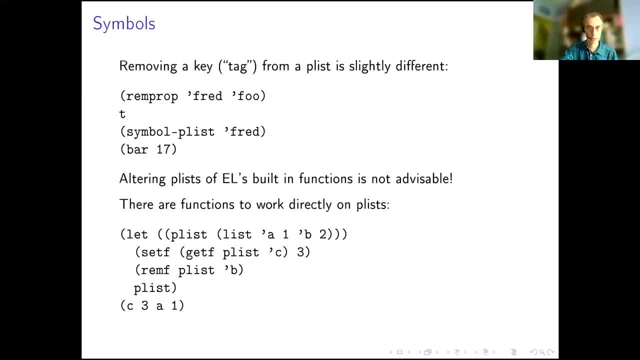 And normally you wouldn't need to look into the playlist yourself, but you may want to because You are trying to Declare, debug something, or or you're trying to find out why emacs treats your symbol is something special. There are also ways to remove. this goes back to a really- it is really- ancient list. so so there are lots of. 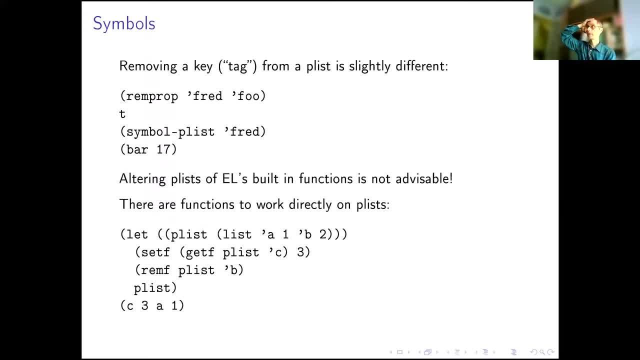 I think in older lists that used to be a put function as well. so you would say: put symbol, key value, And it will then put that into the playlist. now put disappeared from this at some point, so instead we have this set, which: 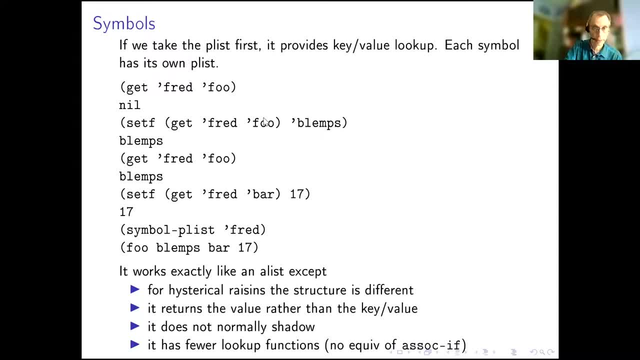 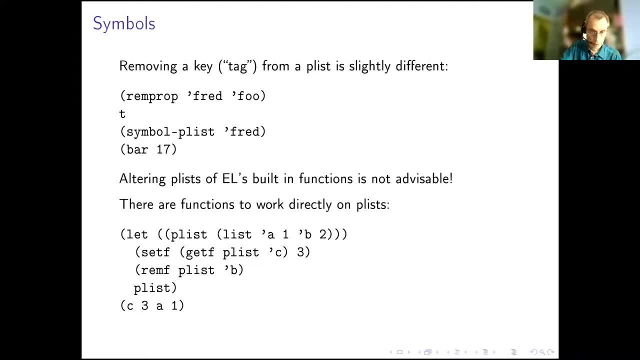 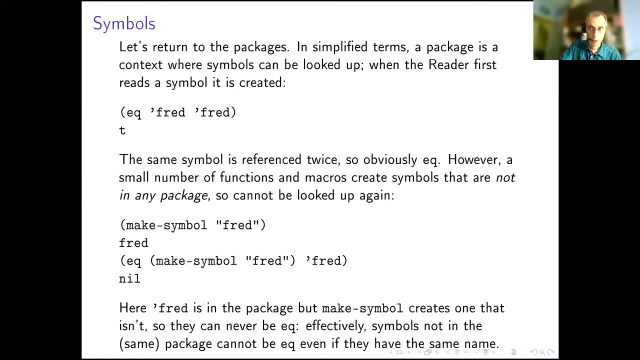 That is indicated by: get the symbol and the key. Okay, So that's it for the P lists. mostly you don't need, you don't need to worry about them, But they can be useful. six: inspect in emacs because emacs makes use of them. if we now move on to the packages that I mentioned, that I wouldn't talk much about and I will say a little bit about it. 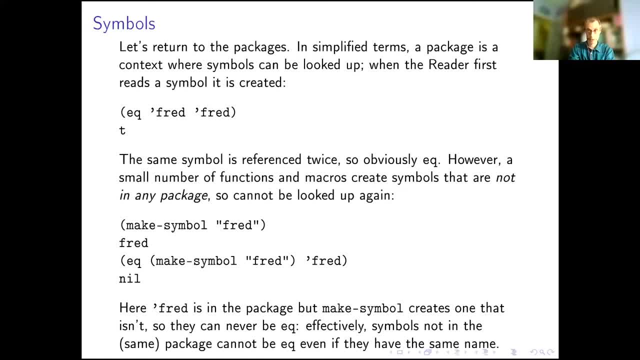 The point is that a symbol is normally in common list is looked up inside of a package. So symbols can be imported into a package, but they will generally always have a home package what Where they belong. So When a common list starts up, there's normally a common list package where all the predefined symbols are car sort, cdr and all those functions, map, car. 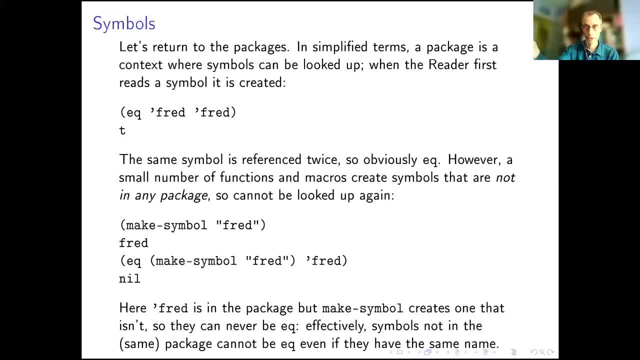 There is a user package where I can create my own symbols and bite The news, a package so I could actually create my own car function in my own package Which, if I do it right, shadows the one in common list and can call the one in common list. 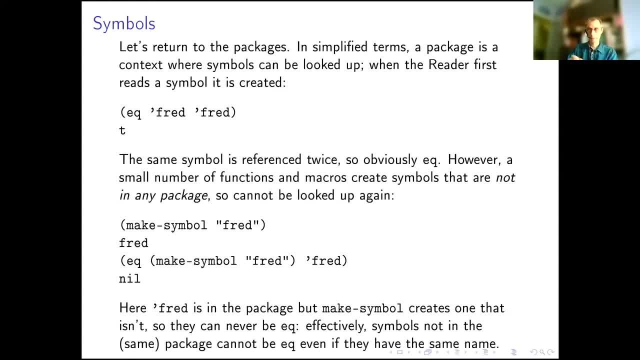 If I wanted to, because they they will not conflict with each other directly because they will be in different packages. The point is that a symbol is referred to as its name When you are within a particular package. Emacs, as I say, don't doesn't really have packages, but it does have. 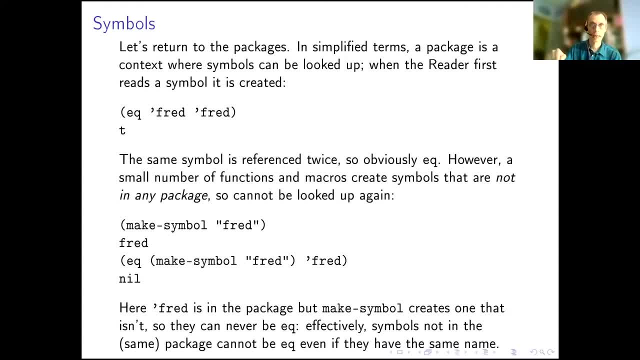 Some key words and things and essentially keywords, are a package of its own kind and there are things in emacs that behave a little bit like packages. So The other point to remember about packages is that most simple secret that I create by saying makes, if I say, if I take a look at the package, 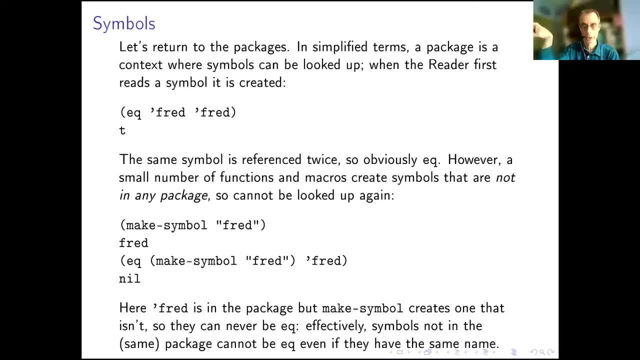 And If I take a look at it, If I take the lessons fred, it will create a simple called fred, if it doesn't exist already, and if it does exist, it will return the same simple that I that I meant before. it will be the same simple every time. however, when I said, make simple, 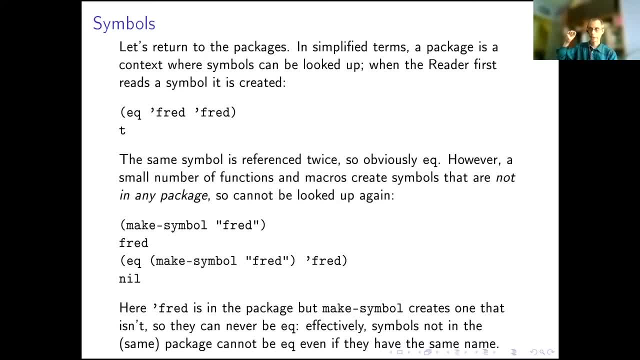 And then pass the string thread in, it actually creates a symbol that is not in any package at all, Even in the max Now, even if it doesn't have packages, but still the simple doesn't have any Home package at all. so the simple, when I say make simple fred, it creates a symbol with the name fred but it's not in a package, so it is not equal to the fred that I can, that I can reference as a symbol. and if I type make simple fred twice, 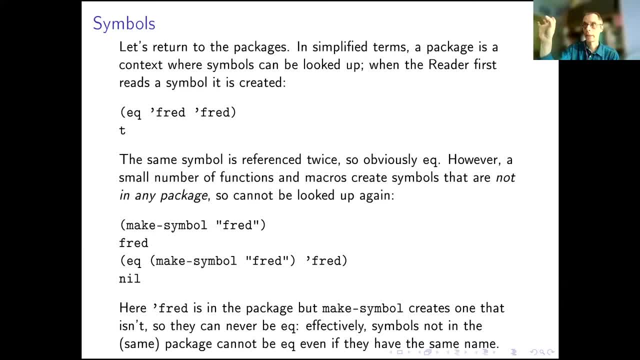 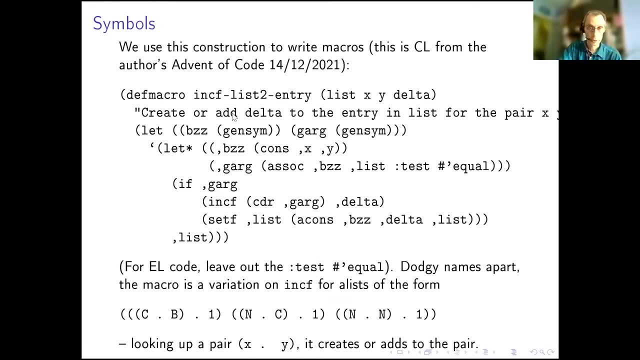 they're still different symbols. In other words, when I use makes simple to create it And, except by a very simple special syntax that i'll show you in a minute, So I can actually use that. so if this isn't a piece of code that i've extracted from one of my 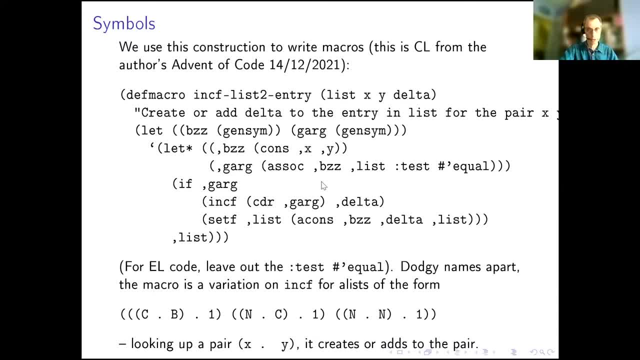 Advent of code or some such it. it updates the list using some sort of by counting numbers of pairs that it encounters And, as you can see, i've used gen sims to generate temporary symbols That are not referenced by anything else, which is useful in. 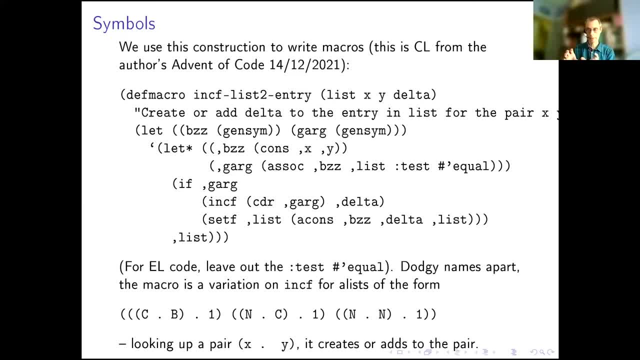 macros, because even if the stuff I want to call is inside of them, It doesn't matter which symbols are used inside of my, the things that get passed into my macro, because I i'm just using gen sims which are guaranteed not to be used inside any other code. 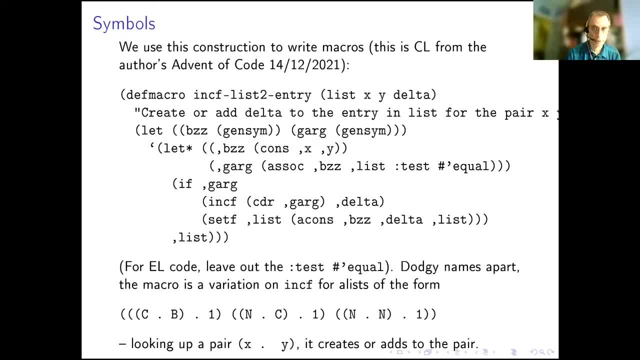 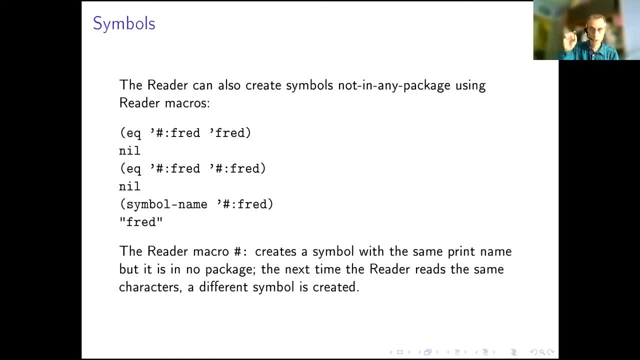 And it doesn't matter so much what this code does. the thing to look out for is the gen sim that i've used here. I can actually use the same thing with make symbols, And I can use make symbols. I can get the reader to make symbols for me. 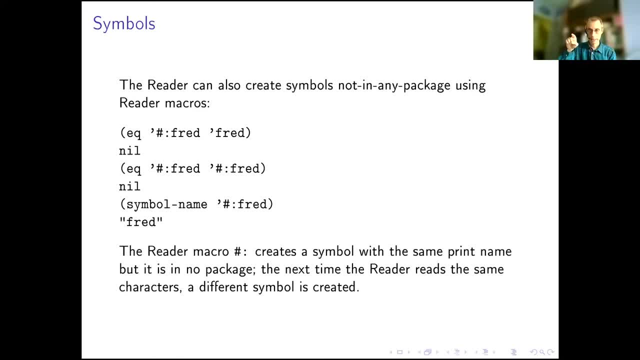 Using a special reader notation that uses the quote hash colon and then Fred. it creates a symbol for me with a print name thread, But it's a simple that is not in any package, just like with make simple, And I can use that in my macro and actually the macro. 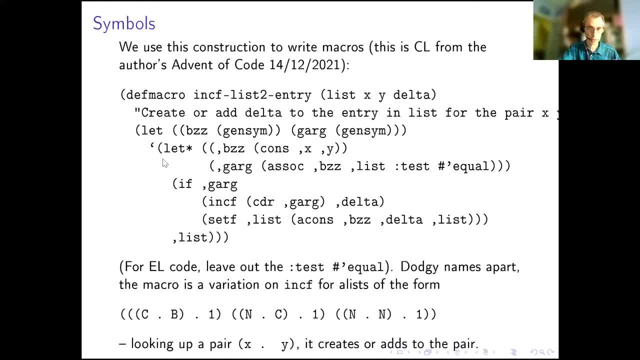 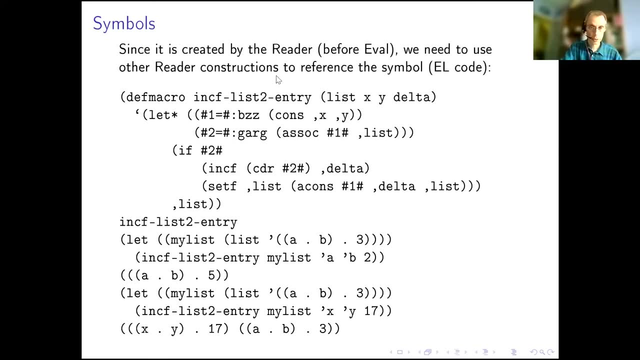 Get shorter now because I don't need the. if we go back for a moment and see: so I had this lead That creates the gen sims and remembers the values of the gen sims and of the second. could have chosen more sensible values, But this thing uses a special meet reader: macro hash one equals. 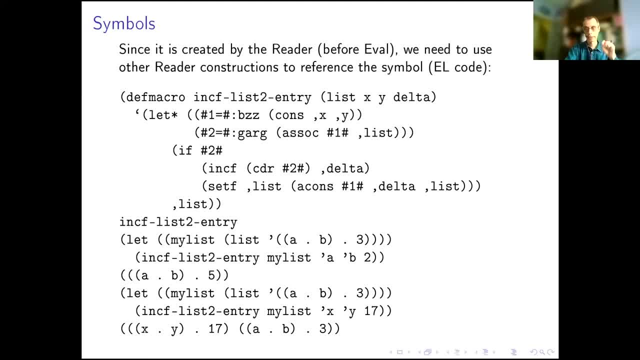 And then hash colon, these. that said, that creates a symbol who's print name is bzz, But it's not in any package. it can never be referenced again except using hash one within this particular call, within this particular set of parentheses. So it creates a simple way. 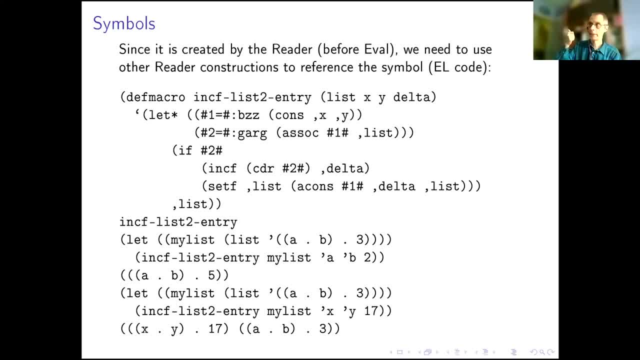 As as if using make simple- except it's not created during evaluation- is creating, created by the reader when it reads this code and it remembers that it's seen it and So that's simple now because it's not in a package And the reader remembers that it's seen it by this hashtag on it and can references and in the code. 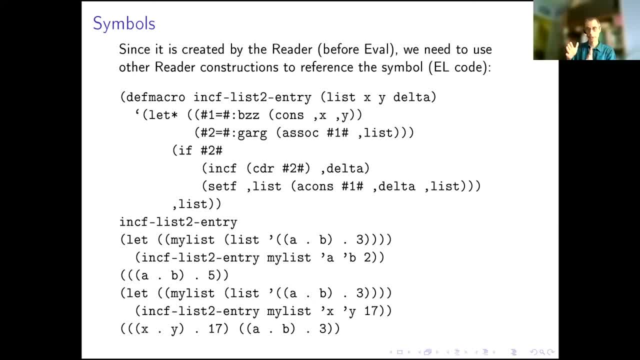 And if you can get your head around that, Then you can see that this macro is much more concise because it doesn't have that lead layer around it. so it actually becomes a nice way to write macros That have unique symbols that are guaranteed to not. 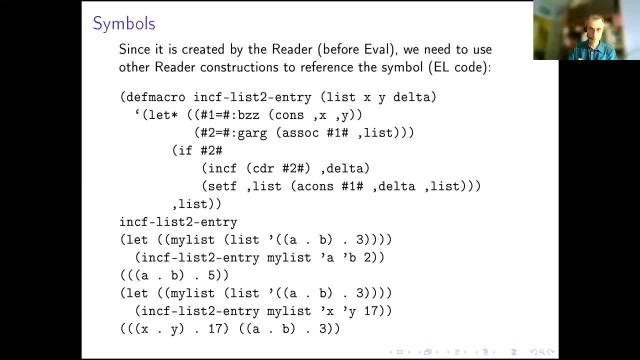 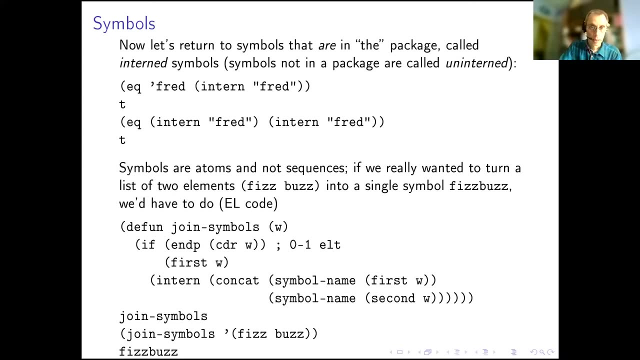 occur in any code that you can pass into the macro, And it also shows how powerful the reader is, because the reader can do lots of things that would otherwise happen at a value, if at evaluation time. So What happens then if I want to create a simple and over- running late, but i'll wrap up shortly. and what happens if I want to create a symbol where I am given a string and I want to have it in my package? 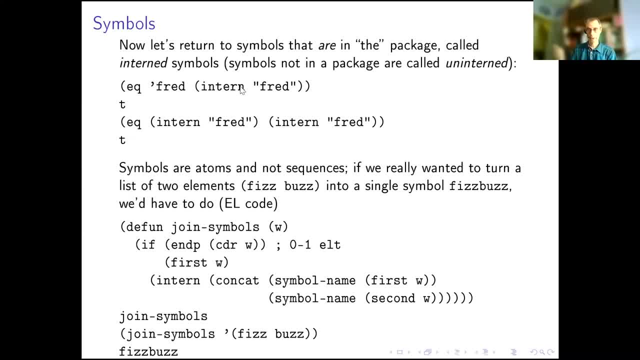 Then I use the intern function. the intern function creates a symbol where the same name, the same print name And it is in my package so I can look it up, my name. So, for example, in my fist buzz code, if you remember back to that, we had the symbols fizz and buzz returned by the, the whatever request into that code. 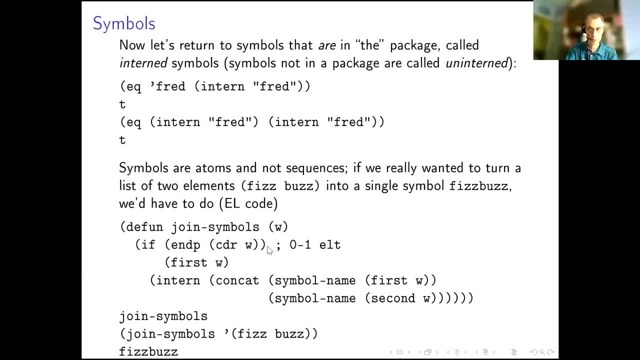 And if I wanted to do to do that by joining the symbols, Then I could actually convert the symbols into strings, concatenate the strings and then convert the string back into a symbol, which is a little bit clunky, but it's entirely possible. 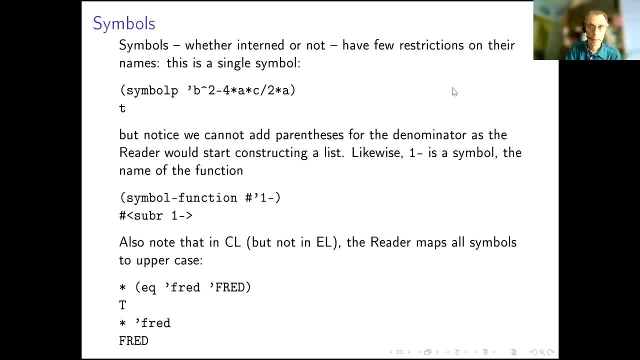 This is my last slide for today and we'll be wrapping up then. so symbols in list have very few restrictions. the one of the few restrictions you have is you can't have parentheses in them, or normally you can't have parentheses in them. 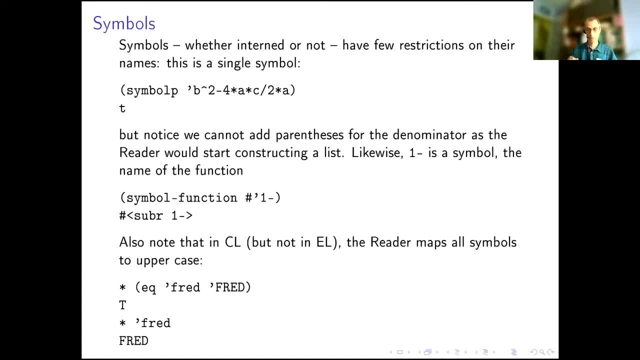 emacs does not map the case of a simple come on, this does. every symbol is mapped, mapped to uppercase by the reader, unless you tell it not to. so Just a compatibility note, because emacs will not change the case of a symbol when he tries to read something. so 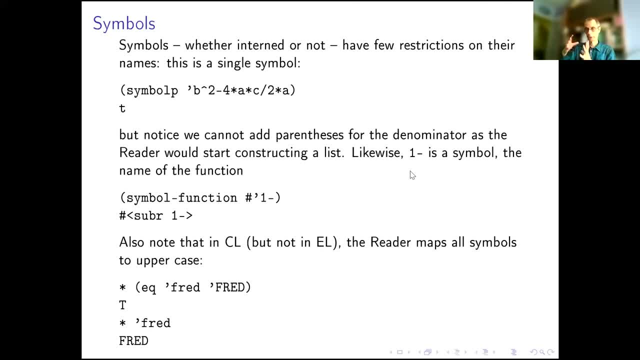 yeah, so simple. it's actually very powerful. you can even put sort of Asterisks and slashes and stuff into symbols if you feel the need for that. this be squared minus four. AC, divided by two way, is a single symbol, indivisible. there are no individual components inside. it is a single symbol used by list. so